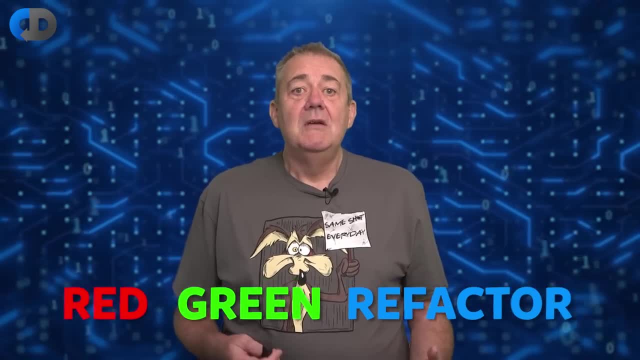 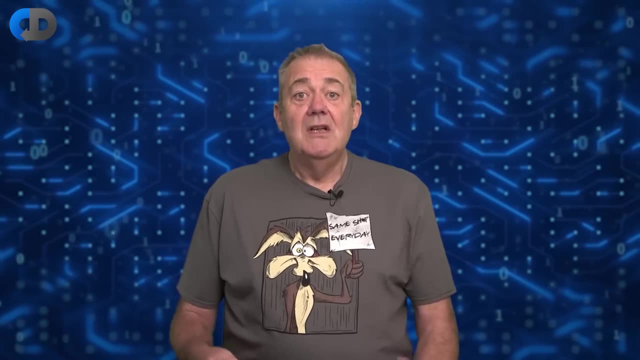 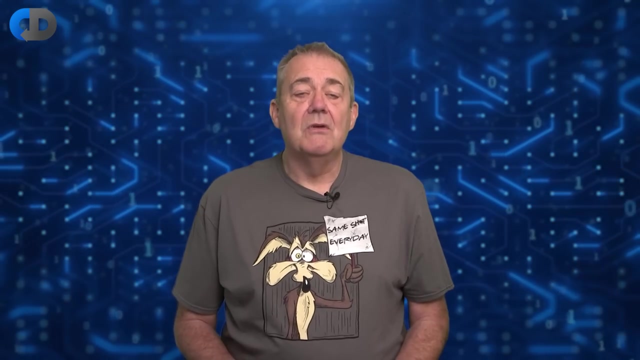 The practice of test-driven development is actually fairly straightforward, but despite this, test-driven development is difficult to adopt. I think that this is for several reasons. Sure, test-driven development is a bit more complicated at the edges of our system, where it interacts with the world via IO devices of some kind. It's also difficult to retrofit to. 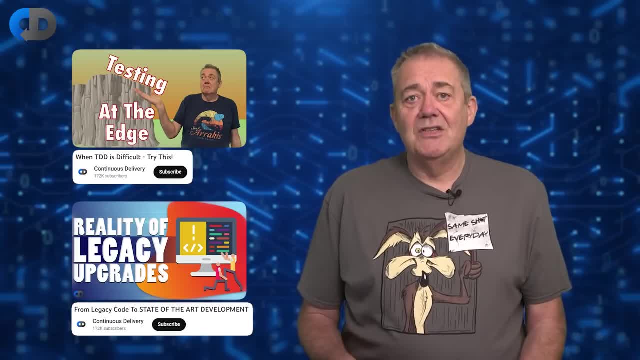 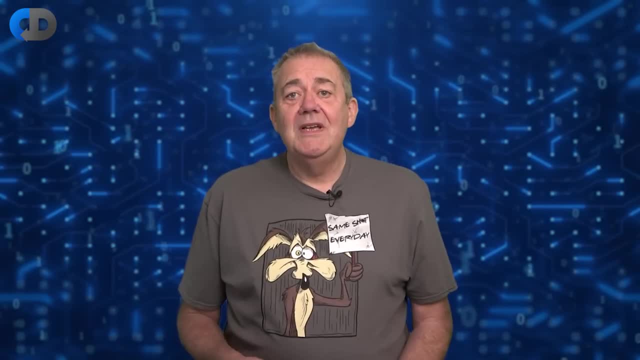 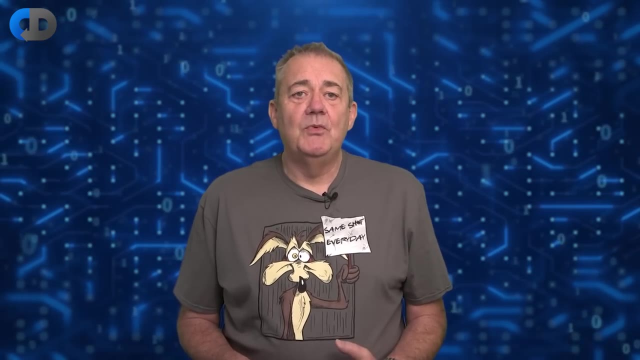 pre-existing code bases, but there are some common strategies for dealing with both of these sorts of things and I've talked about those before. I don't really think that these are the main stumbling block, though. I think that test-driven development works for some fairly deep reasons. but to access 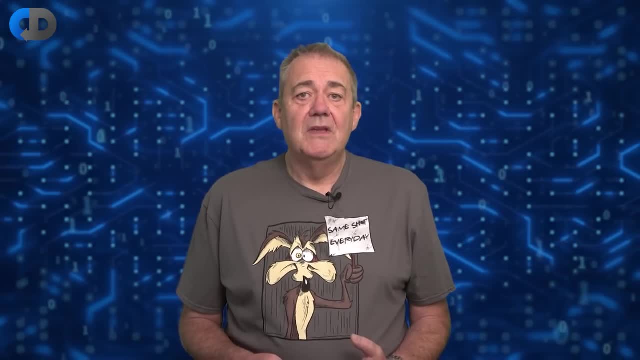 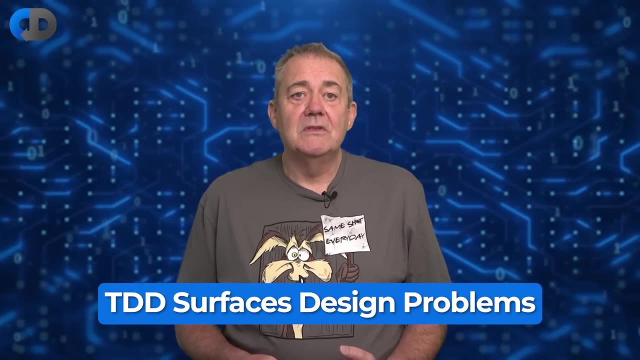 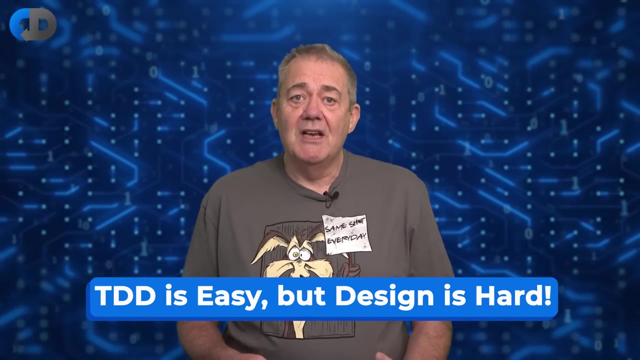 some of these depths. we need a changing perspective. The main problem here is that what test-driven development really does always is to surface design problems. It does this better than anything else that I know, and the trouble with that is that while test-driven development 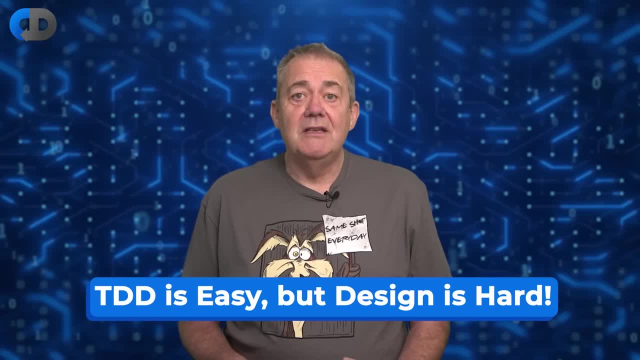 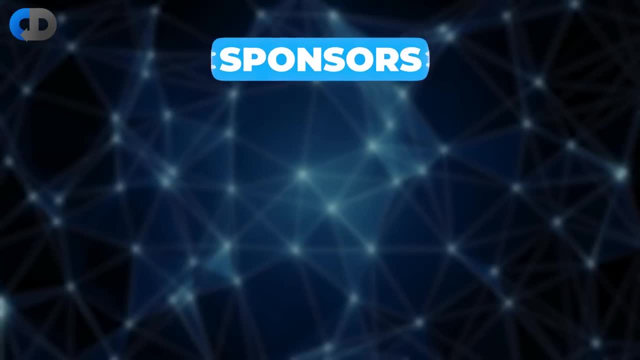 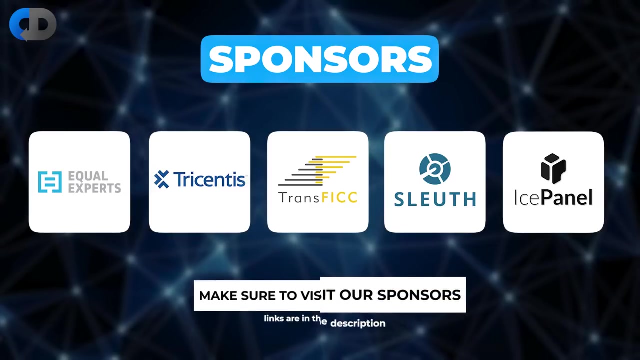 may be easy. design is not Good. design is hard, but it is worth the effort. Let me pause here to thank our sponsors. We're fortunate to be sponsored by Equal Experts, Tricentis, Transfix, Sleuth and Icepanel. All of these companies offer products. 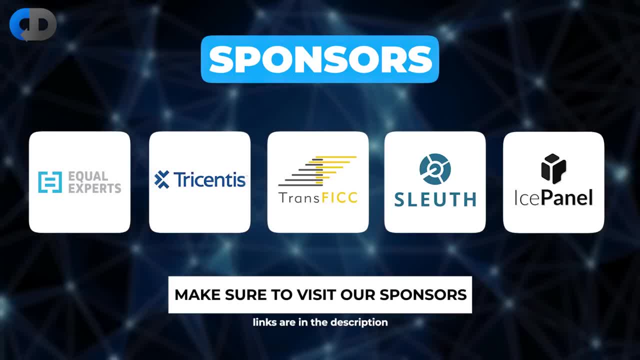 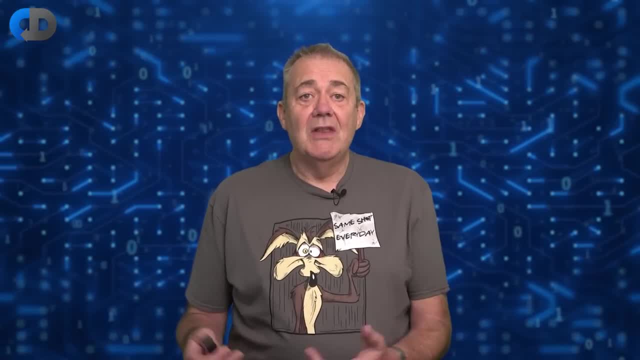 and services that are very well aligned with the topics that we discuss on this channel every week. So if you're looking for excellence in continuous delivery and software engineering, click on the links in the description below to check them out. My impression is that there are. 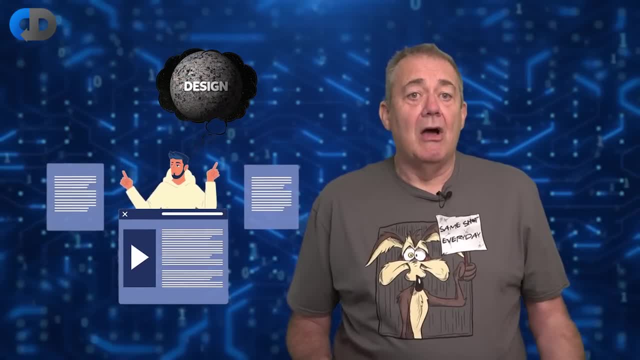 many programmers out there that don't really seem to pay a lot of attention to design and, to be honest, aren't very successful. So if you're looking for excellence in continuous delivery, click on the links in the description below to check them out. All of these companies are very 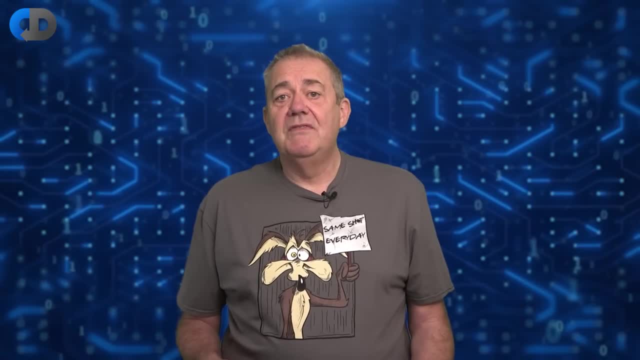 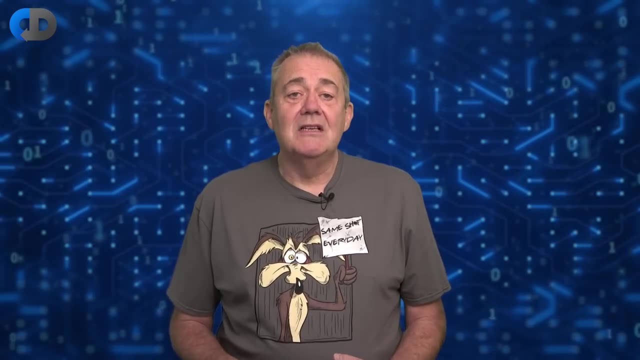 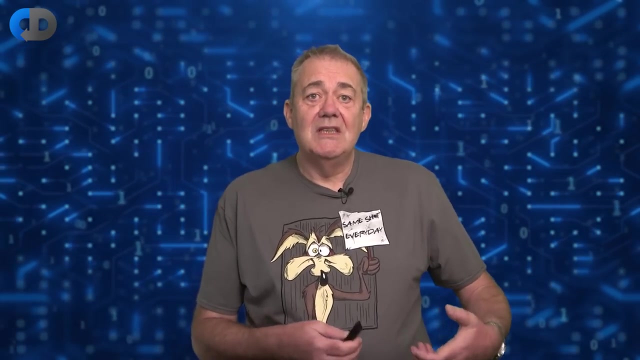 skilled at it as a result. So the barrier to test-driven development is not really the testing, it's the exposure to just how bad their design choices are, and that makes things more complicated. Let's be honest: good design is hard, but TDD helps to point us in the right direction. 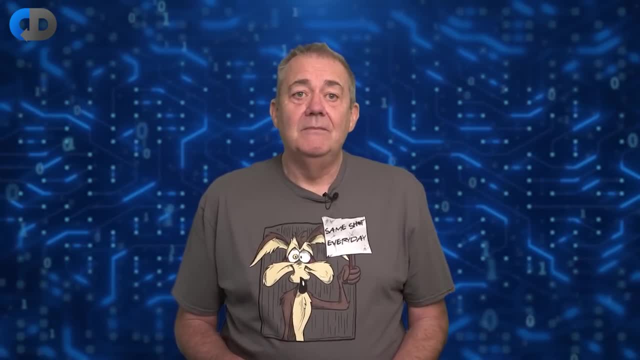 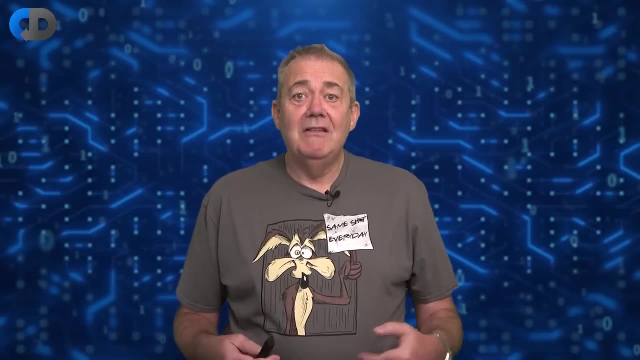 and so can help us to learn, to get better at design. I talk about this in a bit more detail in this video. Don't get me wrong. I value the tests that I get from practising TDD, but for me, the most valuable thing is the feedback I get on my 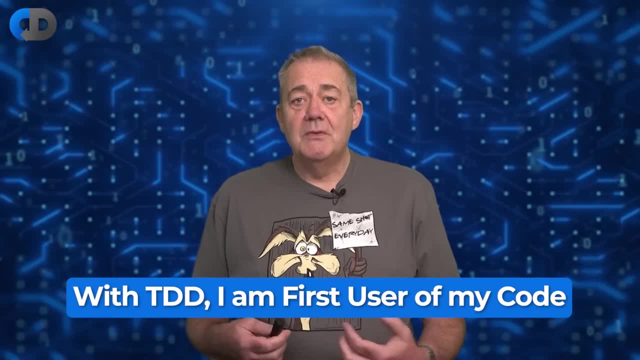 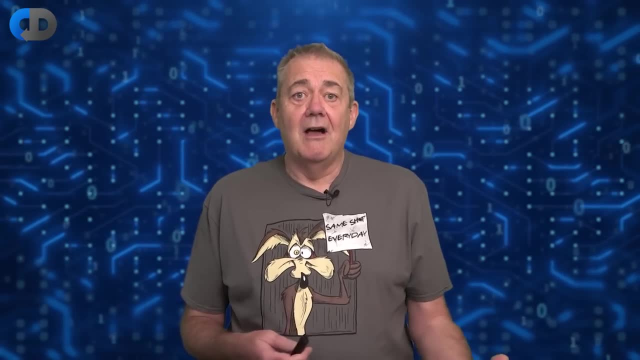 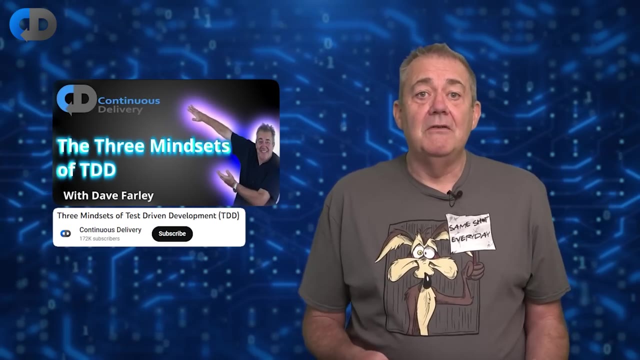 design. I get to be the first person to experience using my own code, and I get that feedback before I've even written it, because I start by defining how I will use that code in a test. I spoke about this process in the first ever video that I made on this channel. 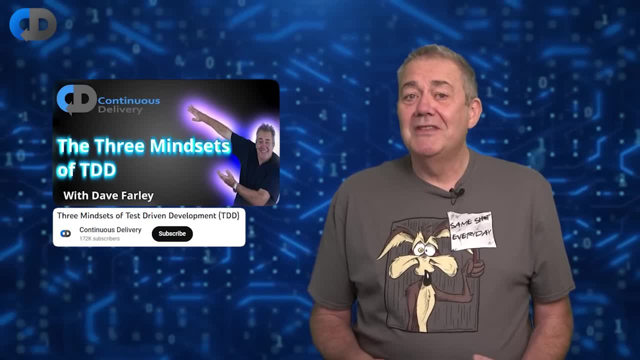 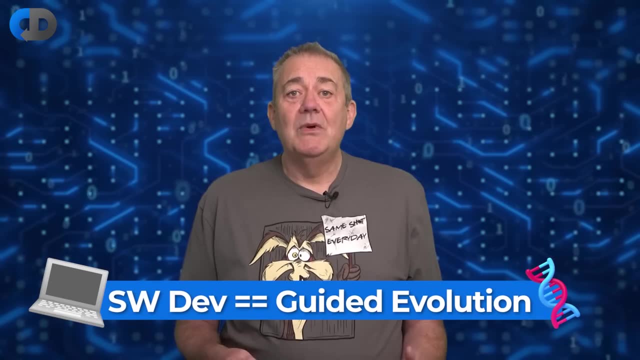 I've learnt a few things about making videos since then, but my views on TDD haven't changed very much. One of those deep ideas at the heart of TDD for me is that we start to see software development as a process of some kind of guided evolution. 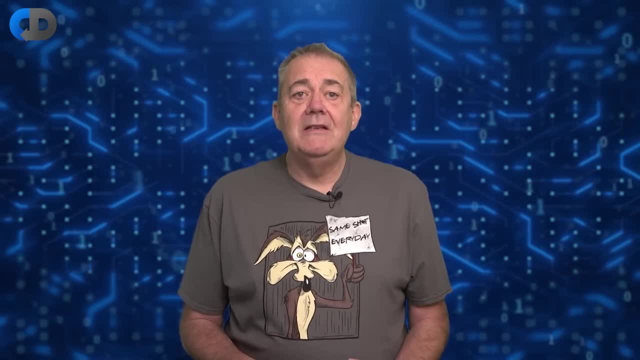 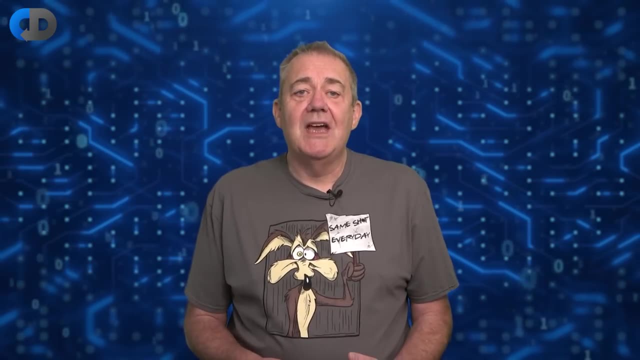 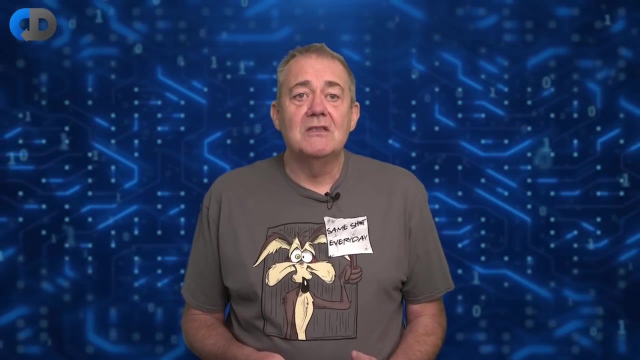 We're going to grow our software incrementally through many small changes, getting clear, accurate feedback on its progress after each small step. This matters. This is one of those, to me, much deeper principles that TDD exposes to us. It frees us to solve more complex problems because we divide them into many small steps. 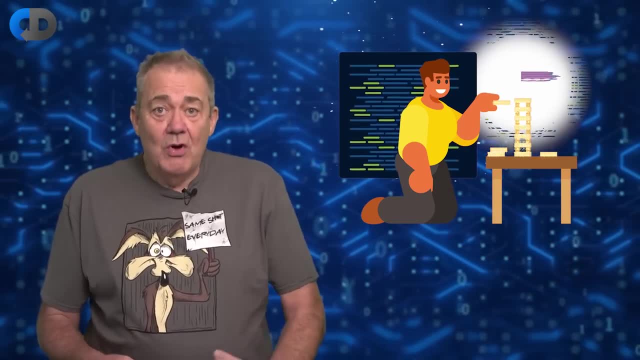 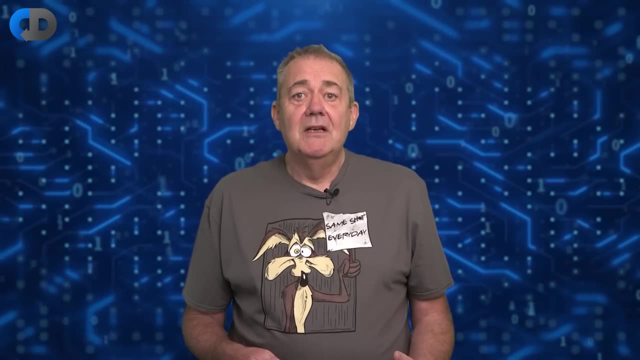 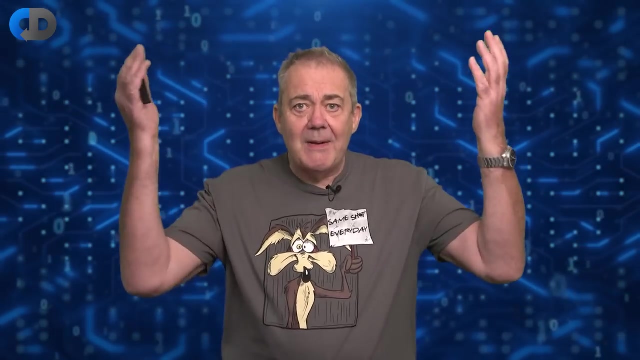 but it also forces us to design in those small steps, more incremental steps. I think that for many people, this is perhaps the biggest and most challenging step from a more traditional way of working to TDD, Instead of thinking hard about a problem. 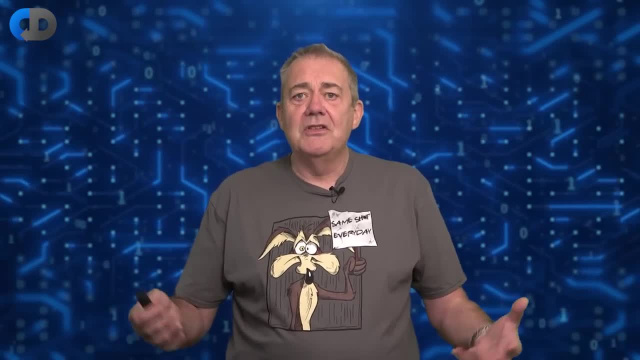 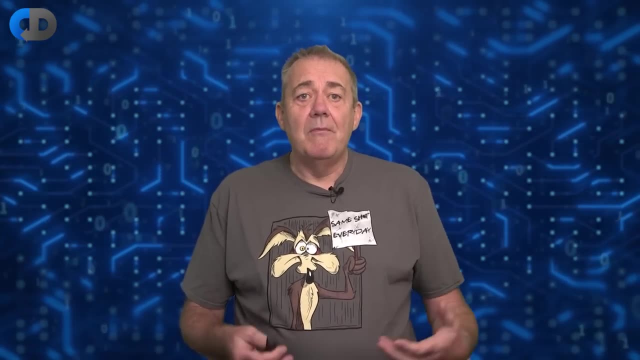 trying to completely understand it and then guessing at a solution that will work and building that solution, which is certainly how I used to work 30 or 40 years ago. we're going to start before we understand the whole problem and certainly before we have the whole solution in mind. 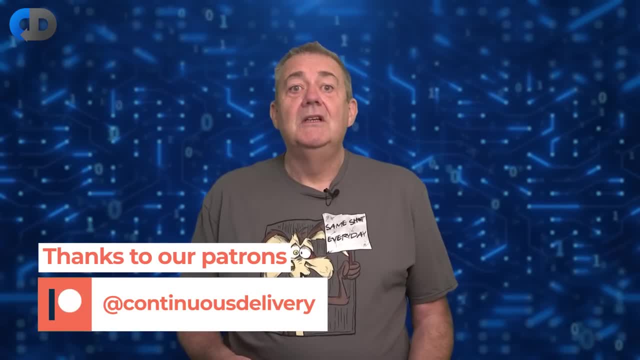 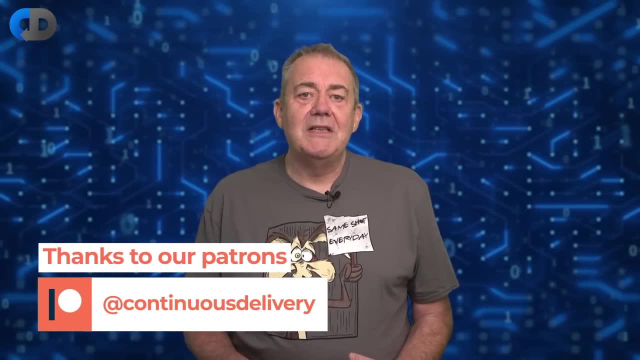 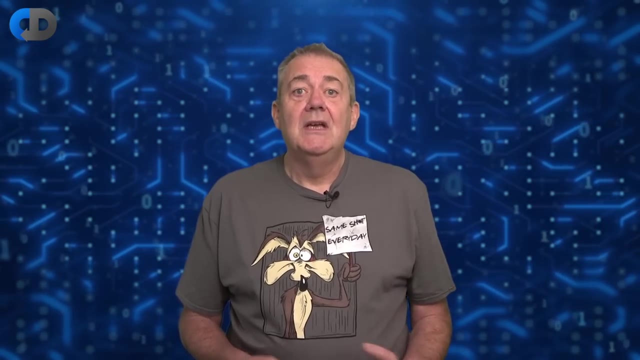 This is a big shift and a bit of a learning curve and I think maybe one of the real barriers that people find in learning test-driven development. The first liberating step when learning TDD is to stop focusing on the solution and testing the solution. Instead, we focus on 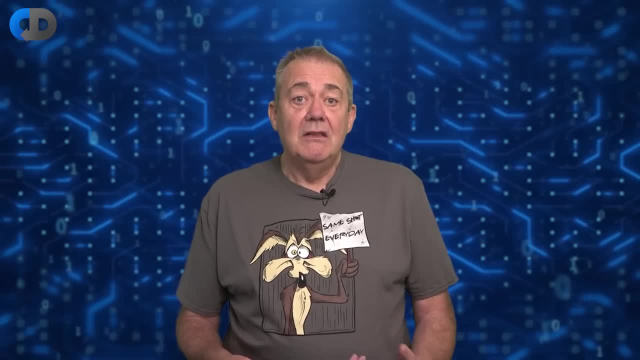 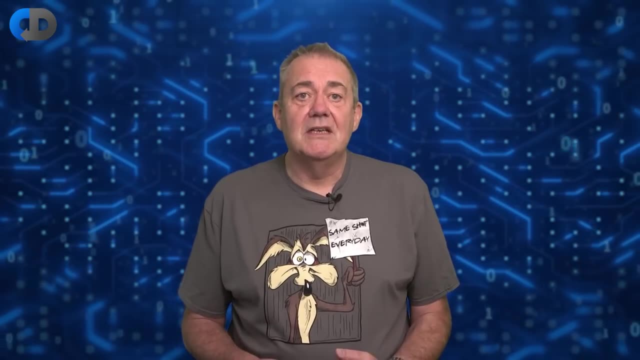 the problem and specifying it in some detail in the form of a test. Everyone makes this mistake at first and imagines the solution in order to be able to figure out how to test it. When I teach test-driven development, I recommend that you consciously avoid this very common 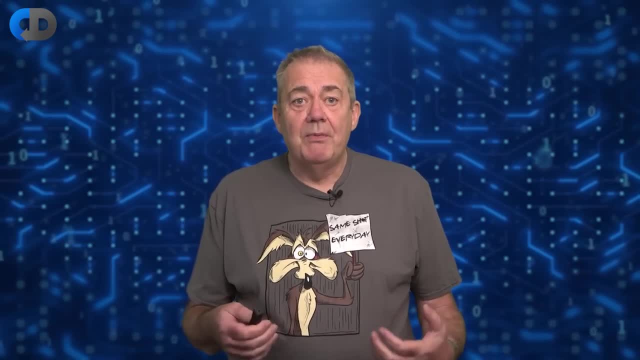 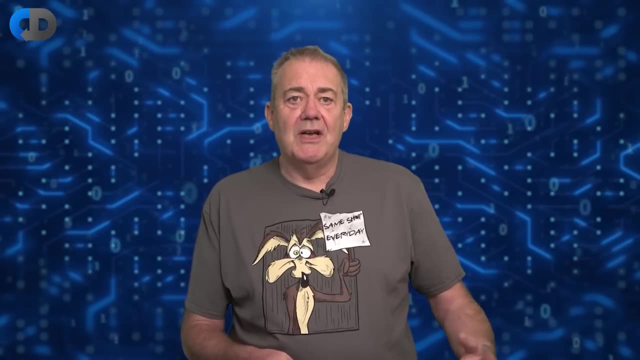 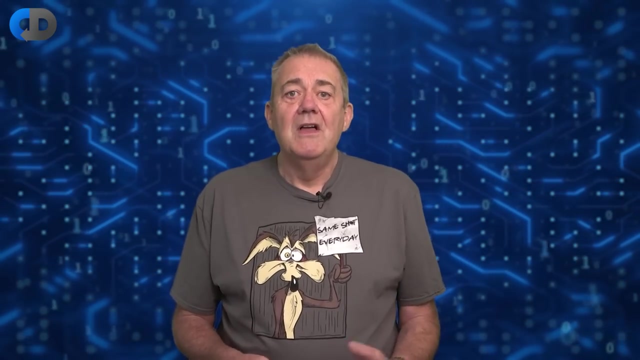 beginner's mistake. Instead, try and describe the problem with your tests and ignore how you're going to solve it. for now, Try and think of a simple example that would demonstrate that your code is doing something useful. Start with the simplest possible case of something useful that you can think of. 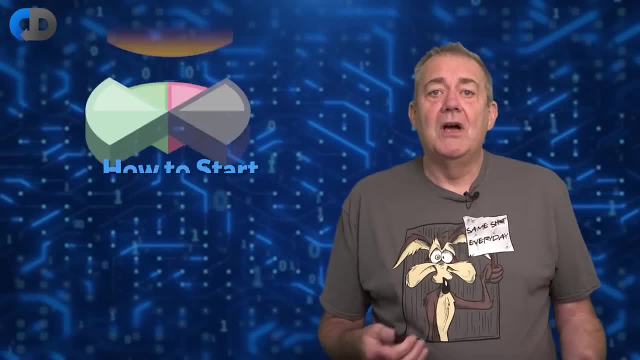 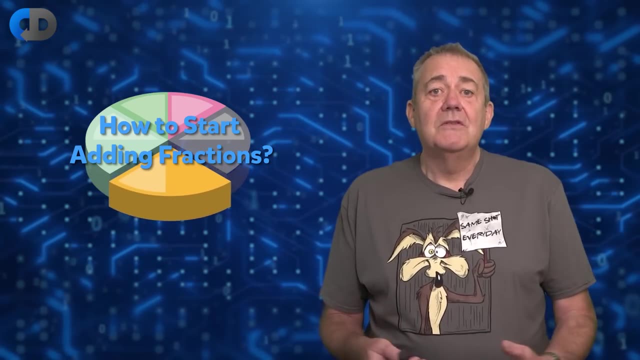 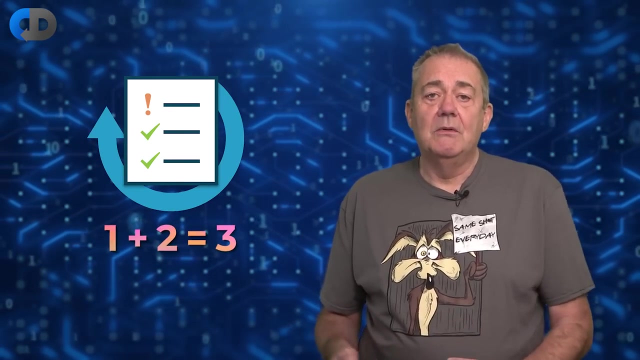 and create a test for that. Imagine we're going to write code to add fractions. The simplest case that I can think of for adding two fractions is to add fractions that represent integers. So I could imagine my first test starting with something like: 1 plus 2 equals 3.. I'll start with. 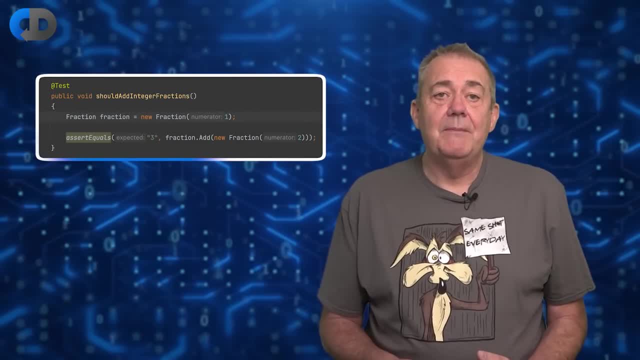 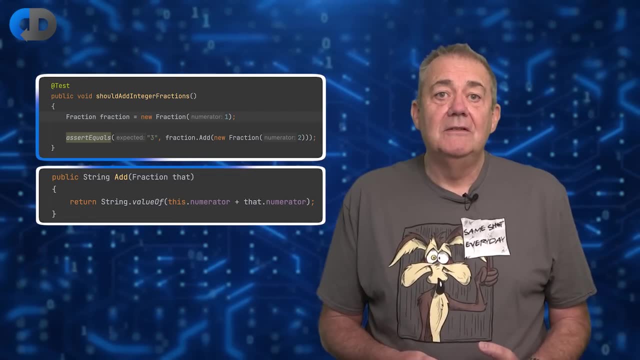 that test and once I have it and have seen it fail, I'll add the code to make it pass. I'm using the creation of this test to explore how I'd like to represent this addition. That's my real focus at this point. 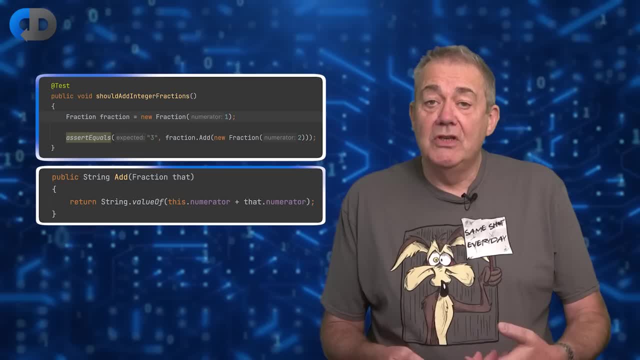 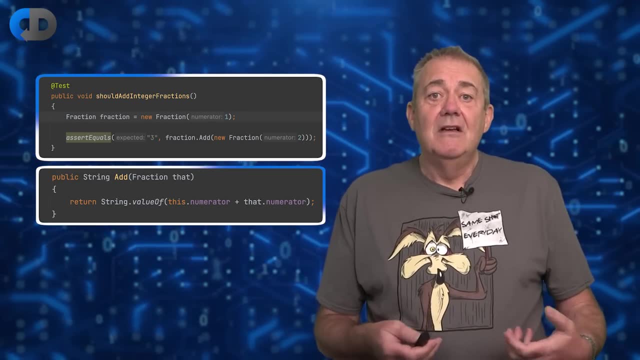 not how I will add fractions, but how someone will use this code, The design of the API to my code, if you like. This will lead me to build a skeleton of my best guess design at this point, with just enough code to make this test pass. 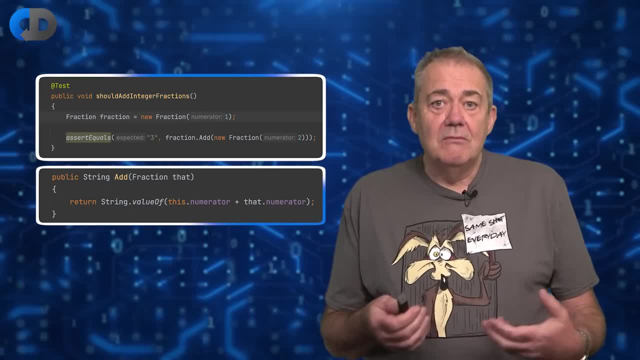 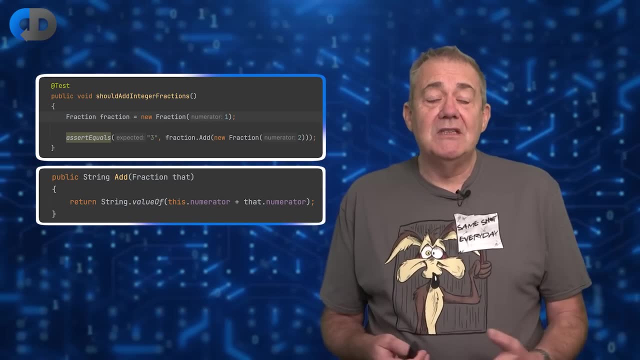 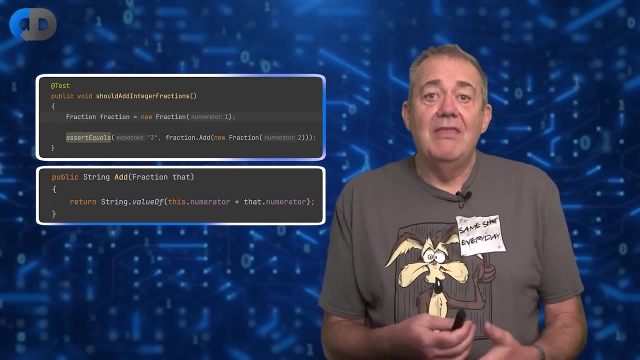 Once all that's working and looking good, I'm ready to move on, but not before. Even at this very early stage, I've already been able to make some design choices. I've decided in this case that I want a type to represent fractions and that when I add 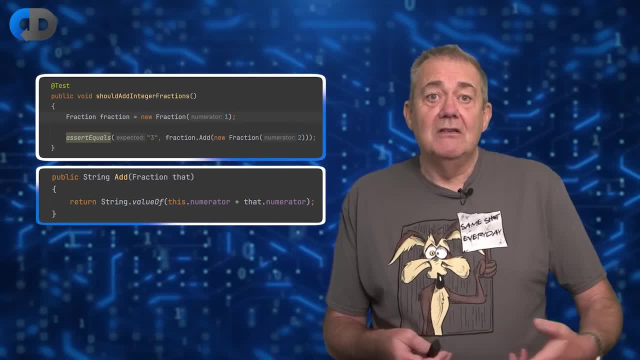 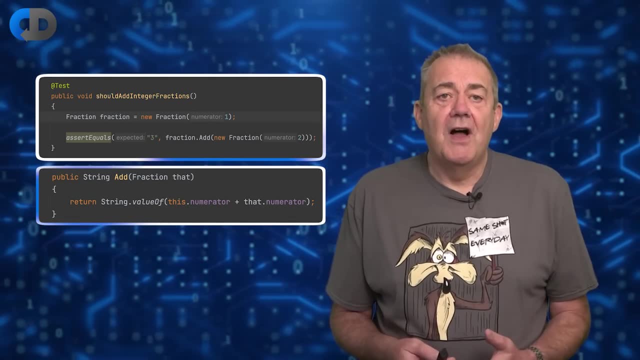 two fractions. I will add them as fractions rather than dealing with them as strings or decimals or anything else. After a bit of refinement, I may refactor my design a bit further and end up with something like this, which is really really, really useful. 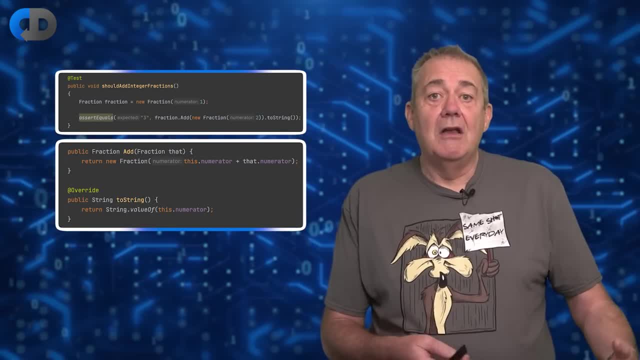 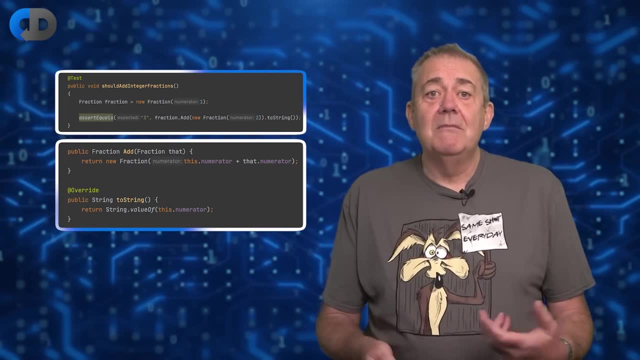 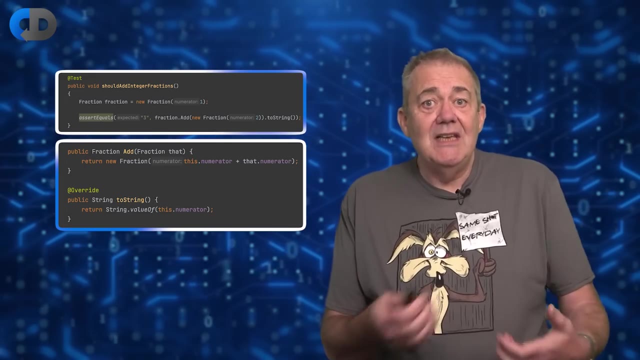 really the outline of my first guess at a design for adding fractions. By choosing this simplest possible case, it's helped me to experiment and play with the basic shape of my code. While everything is at its simplest, I can change it easily and more quickly and make some design choices. and 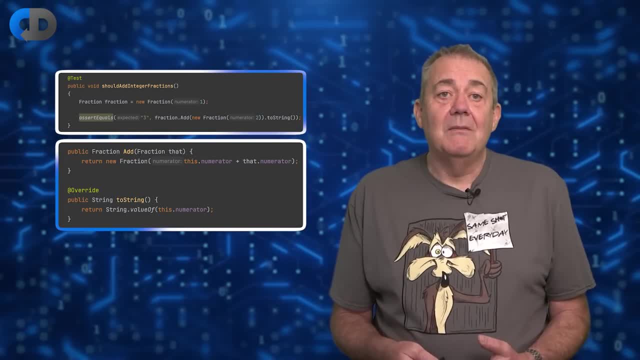 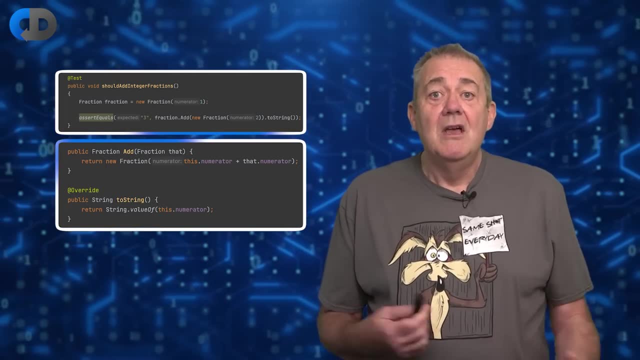 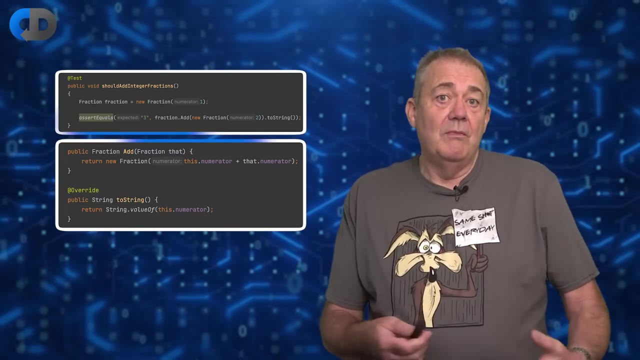 experiment with them. These will shape the next steps. By choosing this simplest possible case, it's helped me to experiment and play with the basic shape of my design. While everything is at its simplest, I can change this code easily and quickly and make some design choices that will help me and shape the next. 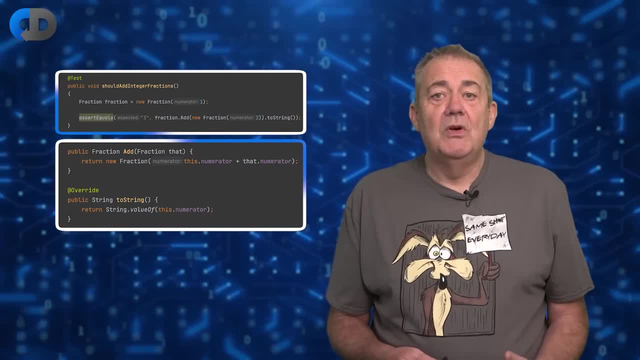 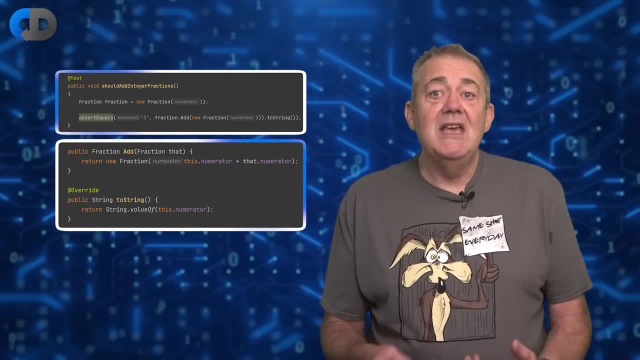 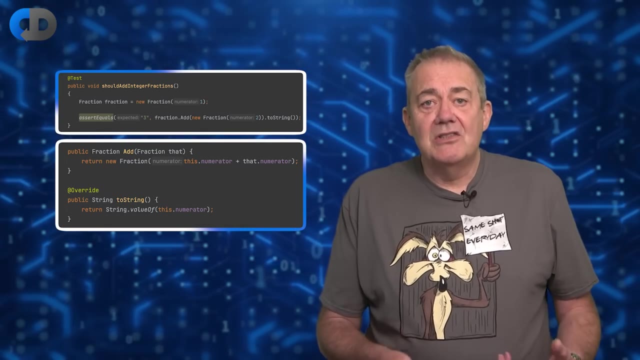 steps. It's not worth agonizing too much over the design at this point, but it's also not worth skipping over it and ignoring this chance. This is the easiest time to correct mistakes or even to explore your preferences. I tend to start reasonably slowly at this point, thinking about the kind of design and 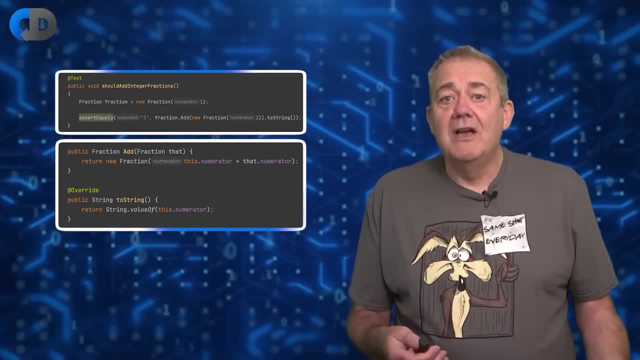 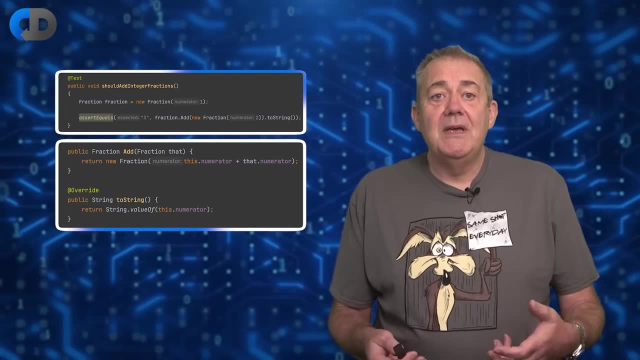 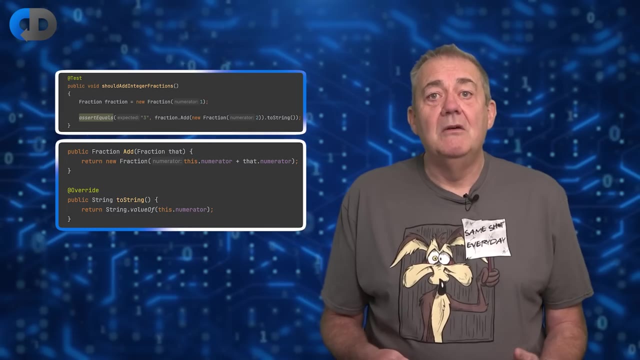 where it might go a little bit, but also trying not to think too far ahead, Maybe trying different ways to organize things. My decisions are being guided by the external usability of my code for this simple case, but also I'm now just starting to think a little bit about some of the broader structural choices. 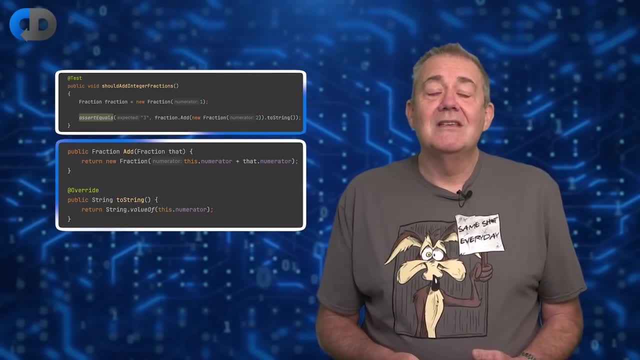 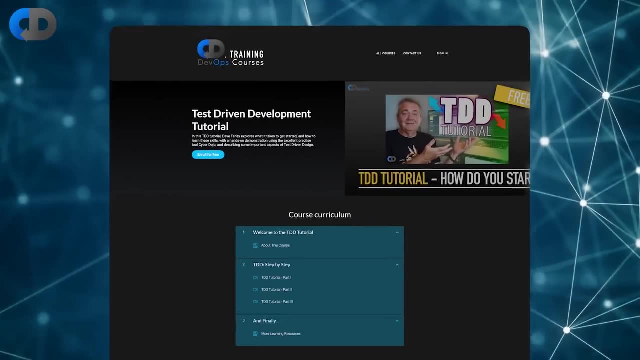 in front of me for my design, This first guess at a solution. If you'd like to learn a bit more about test driven development and maybe try it for yourself, I have a free online tutorial that can help to get you started. Check the links in the description below In. 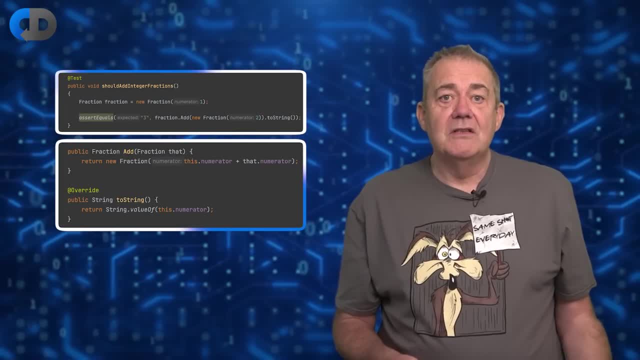 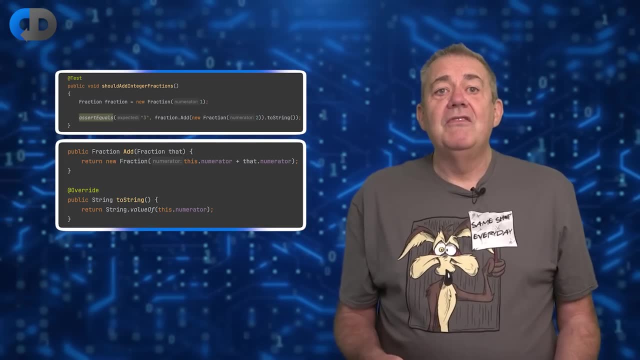 the case of fractions, I've already decided that I'm going to create a fraction type and that to create one of these, I will specify a numerator as an integer, and although I haven't done it yet, I'm pretty sure that at some point I'll be adding another constructor that probably takes 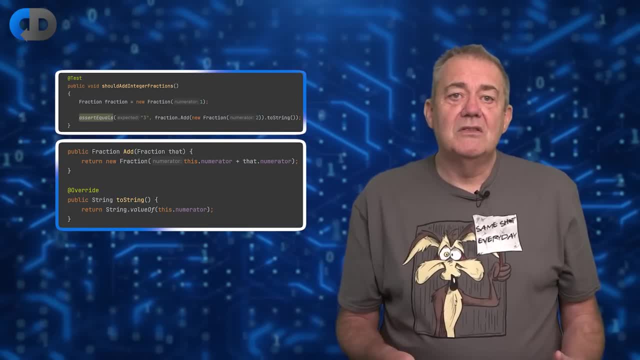 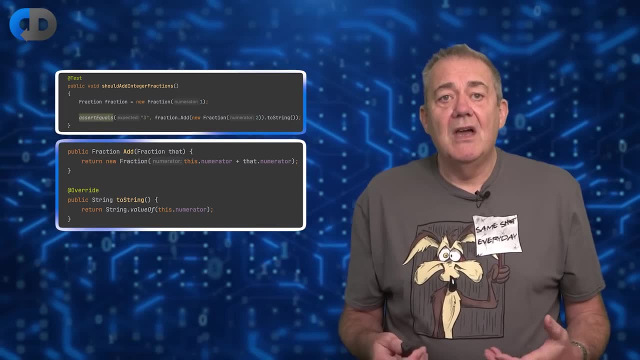 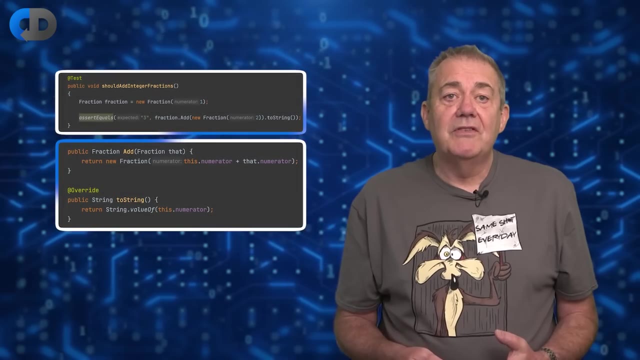 the denominator soon. I've also decided to separate the concerns of addition from that of rendering fractions into a string representation. I used the- the ideas of managing complexity that I describe in my book, as guidelines, even at this simple, trivial level of code. As I said, I always try to imagine the 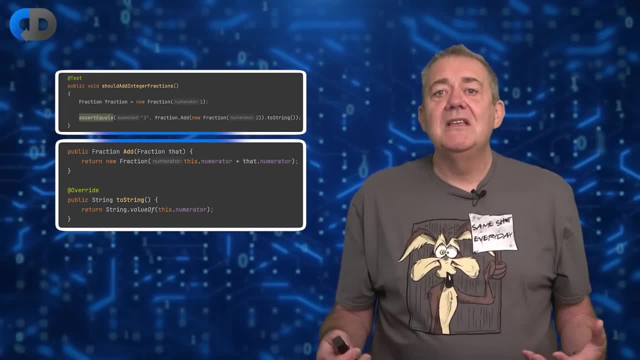 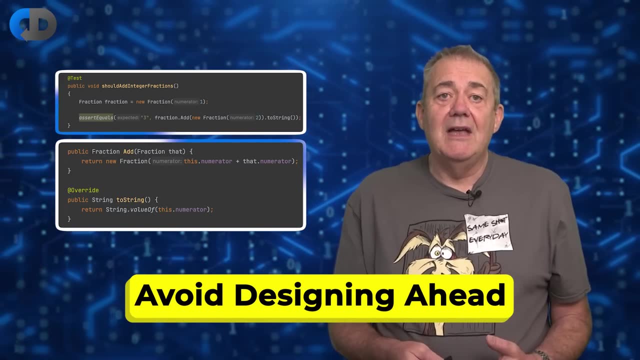 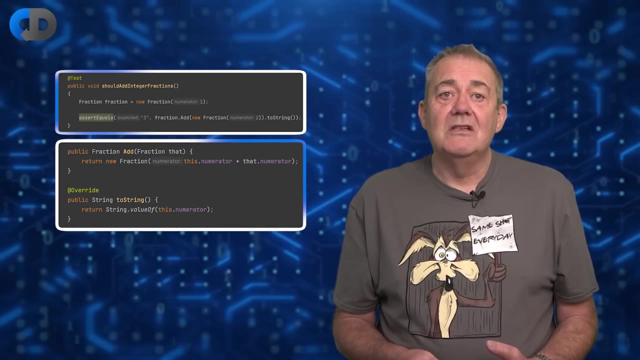 simplest possible case for my first test. I think it's okay to play with this at this time to explore your design, but you should avoid designing ahead. as I've already said, This is a subtle difference. At this stage, I'm only focused on adding integers. I've made some small mental steps ahead. Strictly, this is a risk. 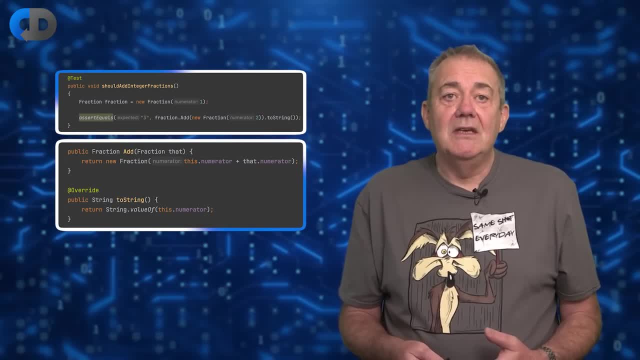 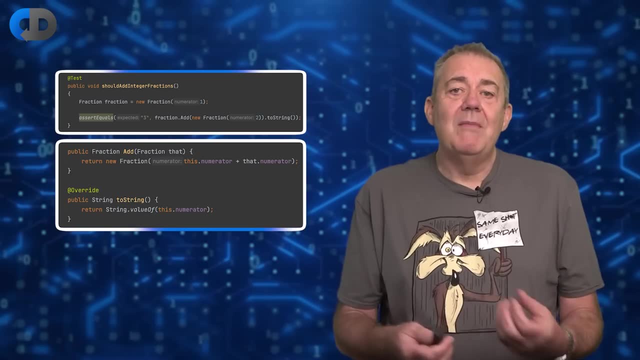 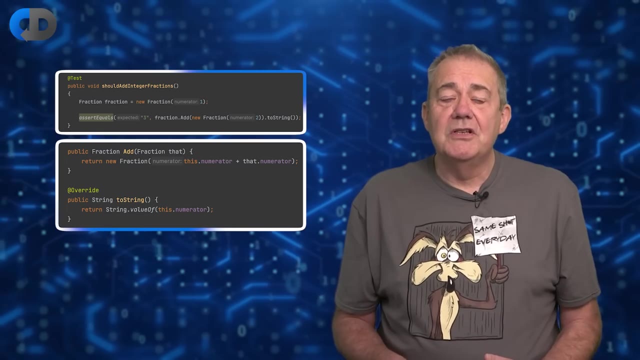 and I'd advise you to be very cautious of steps like these. but I don't really see any reason why I should remove my brain from the process of test driven development. So I'm happy to think ahead, a step ahead or two, but to try and rein in any desire to imagine the solution to the whole. 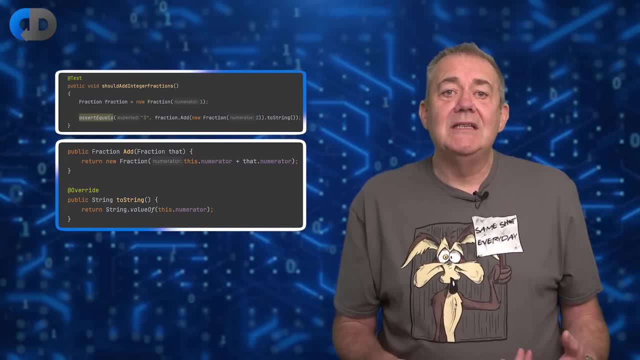 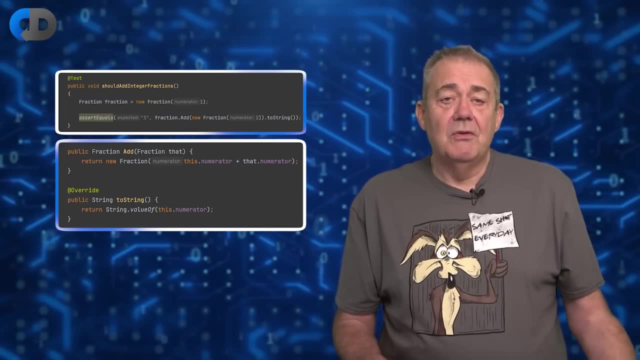 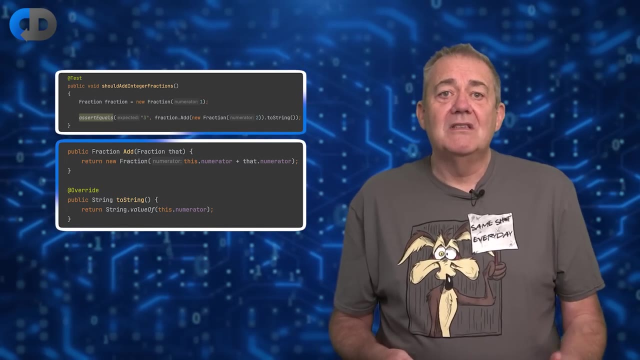 problem. So, for example, if I were only adding two numbers, creating a fraction is really overkill, but I'm not. I'm working on something that I know is aimed at adding fractions, So I think it would be naive of me to start with a test that confirmed that 1 plus 2 equals 3, using only integer addition. 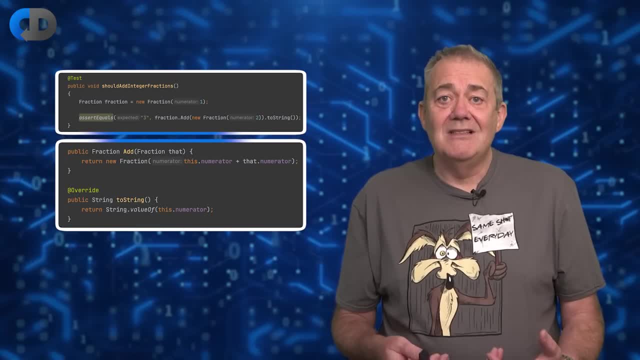 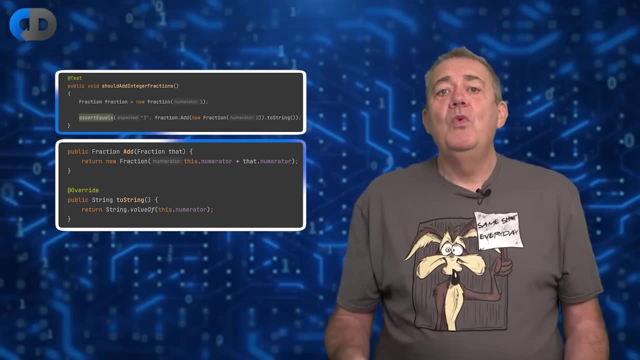 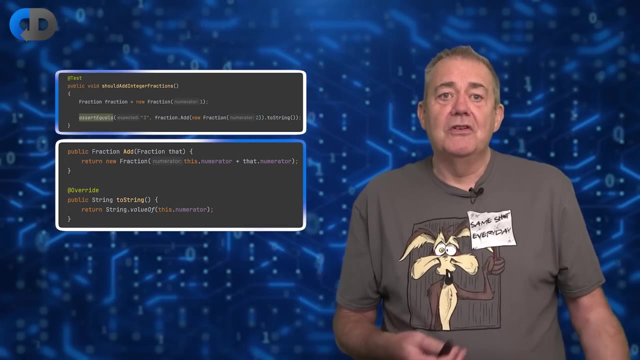 I am, after all, using this test as a design tool, not as a means of verifying that maths or integers work. in my programming language work, I'm willing to believe that those things already work. So the job of my first test is to help me think about how to structure my code for adding fractions. 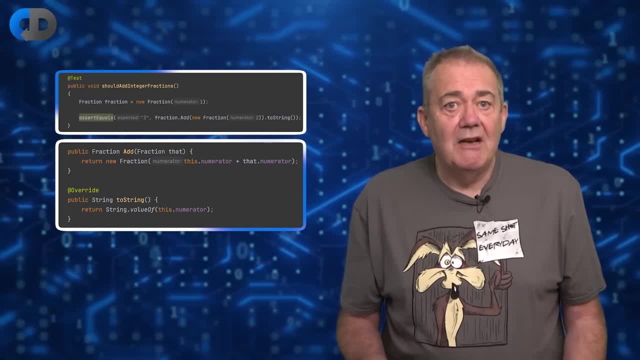 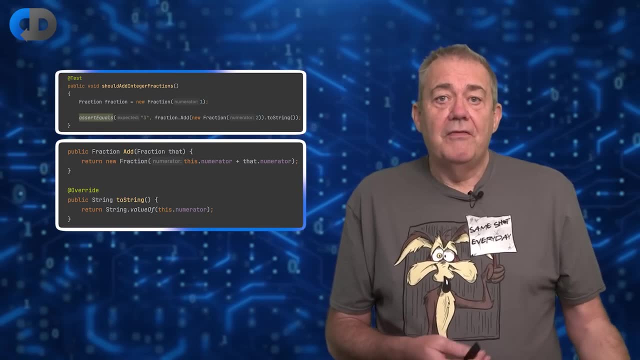 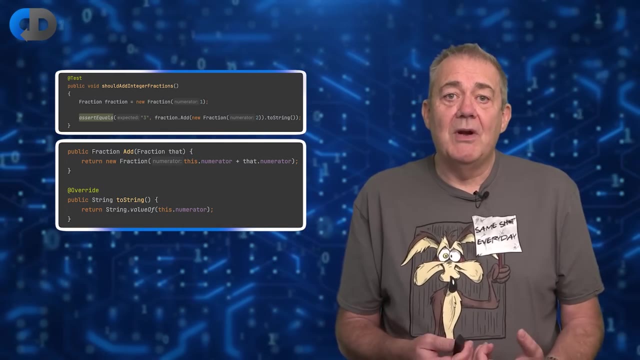 The bear trap- here is particular for beginners- is doing too much of that thinking ahead. Here, I'm comfortable with identifying my desire for a fraction. I'm going to use the fraction type to represent the addition and then, through a very simple process of refactoring, getting to the decision to separate the concerns of the addition from that of rendering. 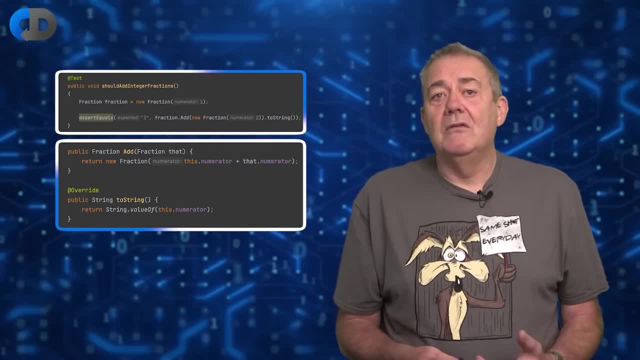 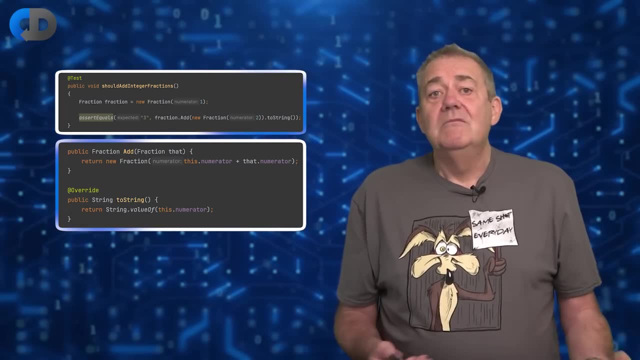 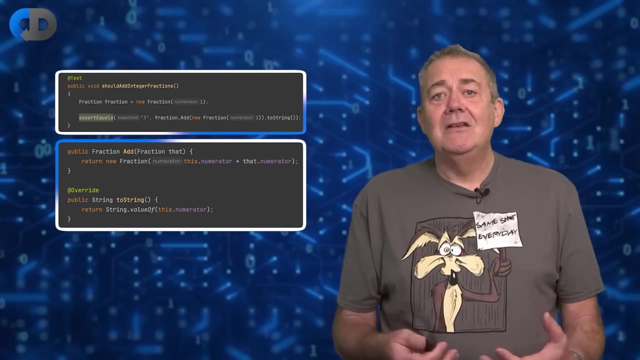 fractions as strings. But you could argue that the decision to return the fraction as a string rather than as an integer or as another fraction is designing too far ahead. I'm relaxed about that additional step in this case, But largely for one reason: At each small step. 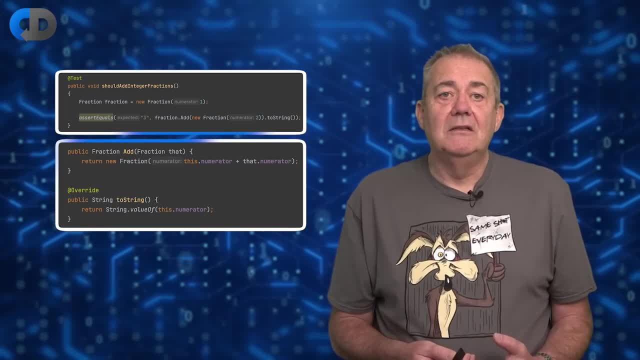 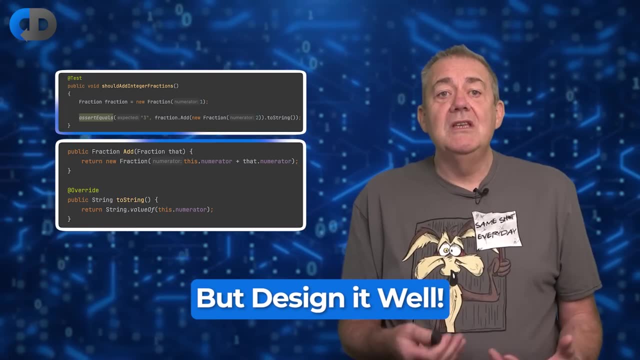 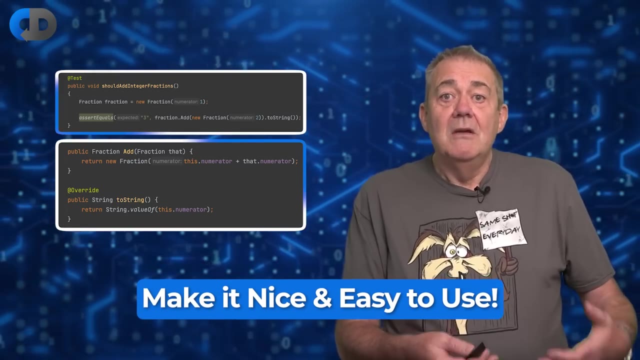 I still want to be doing the best job that I can of my design In the context of the problem as it's expressed in my tests so far and no further. I'm using the test to design my code and specifically thinking about the interface to my code and making that pleasant for a user of my code. I don't want to design too far ahead, but I also count it as a success if my code and tests build up incrementally. I don't expect to get everything right first time, but I also don't aim to write tests that I know I must revisit at the point when I'm writing them. I'm picking tests to advance my design, so I want 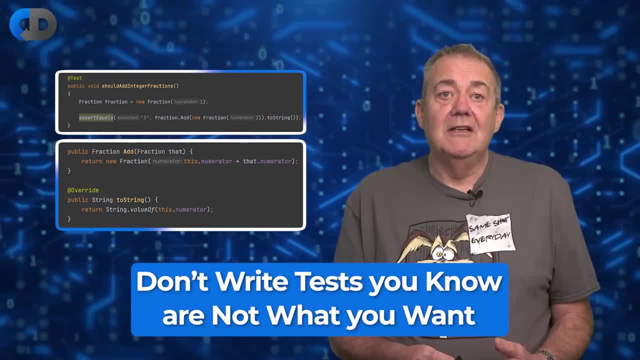 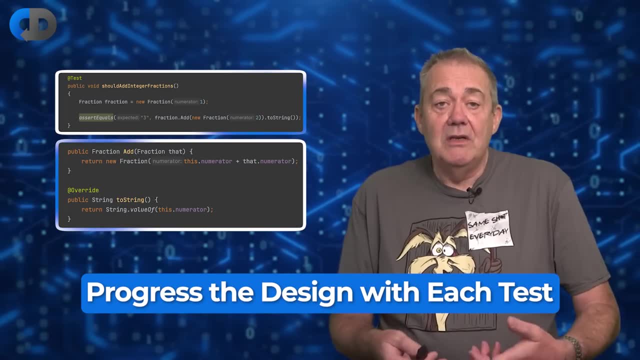 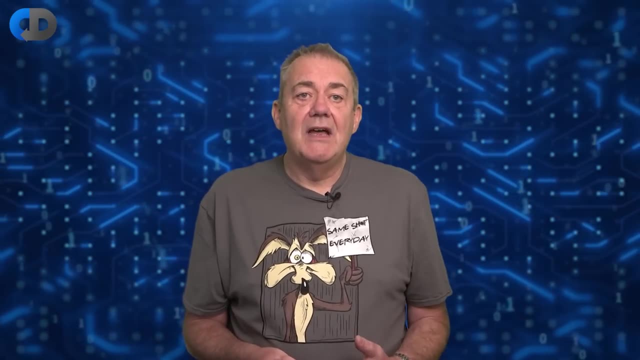 my design to be progressing with each test. ideally. I know that I want to have a string representation and that that will make this test now, at this point, a little easier to read, so I'm happy with that choice. Once we're happy with the first test and the design of our interface, we can start adding more tests. 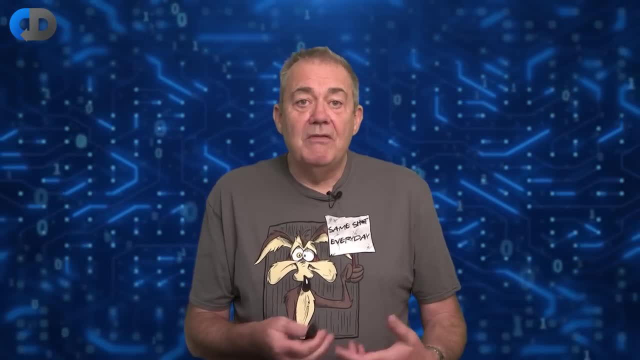 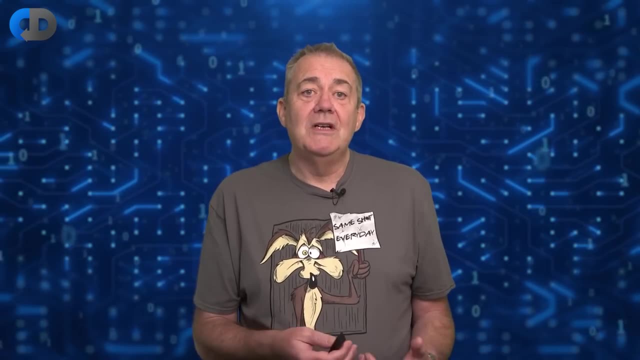 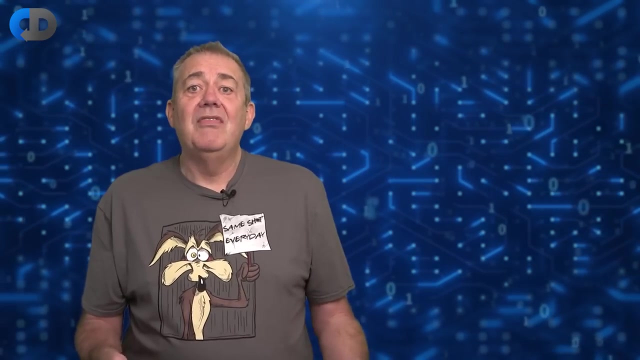 What we want next is a test that will make us explore a bit further into the problem- Not the whole problem, but just a small step and not just a repetition of what we've already done either. There's absolutely no value in terms of advancing our design by testing the addition of two plus. 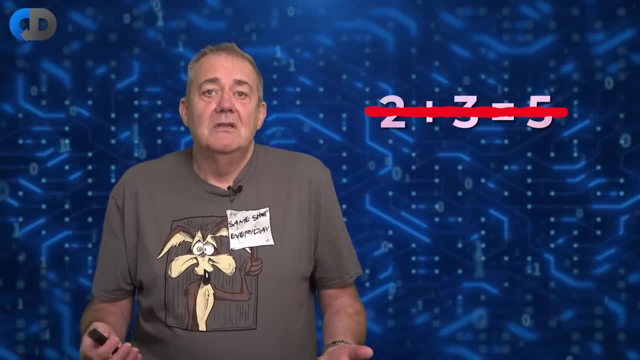 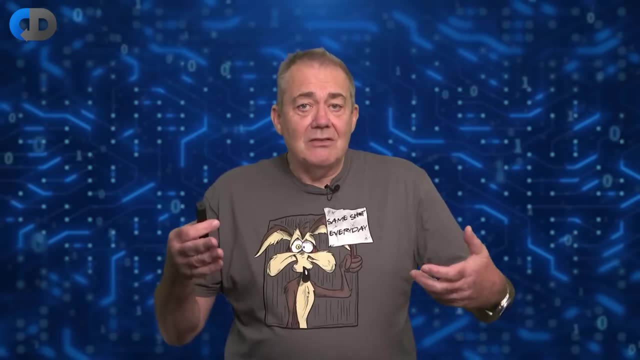 three equaling five, for example. That's just going to be a little bit of work. It's going to pass and it's just testing exactly what we've already just tested. so we want a next step that's not too complex, but not too simple either. Sometimes it can help your thinking to 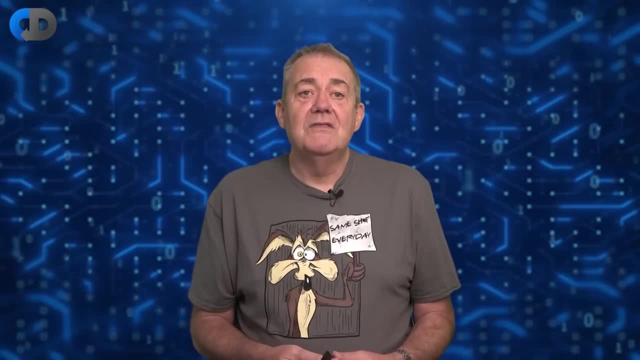 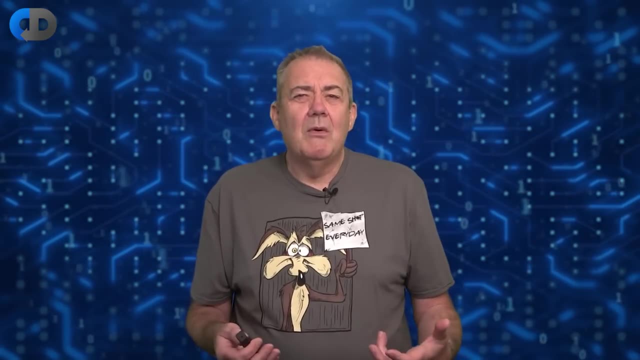 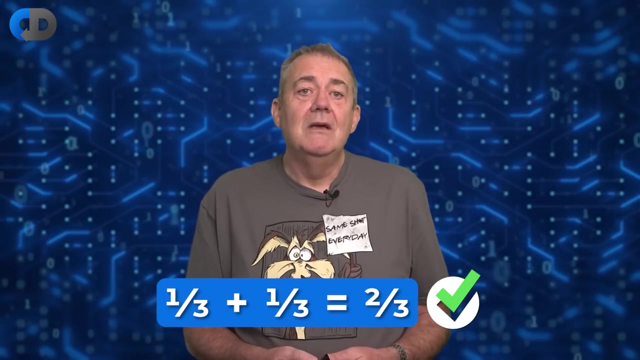 sketch out a few next steps for some kinds of testing For adding fractions. my progression would probably be something like this: Next, we probably want to add some really simple fractions. maybe one third plus a third equals two thirds. This forces us to add that denominator that. 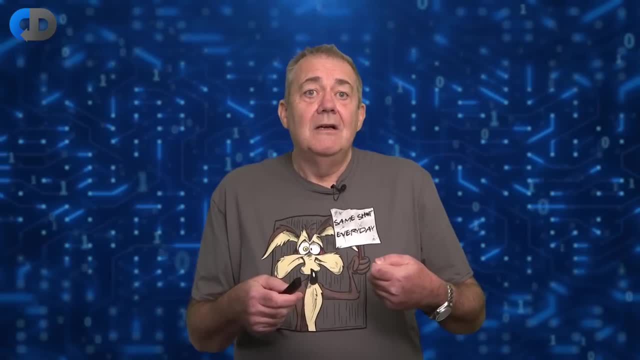 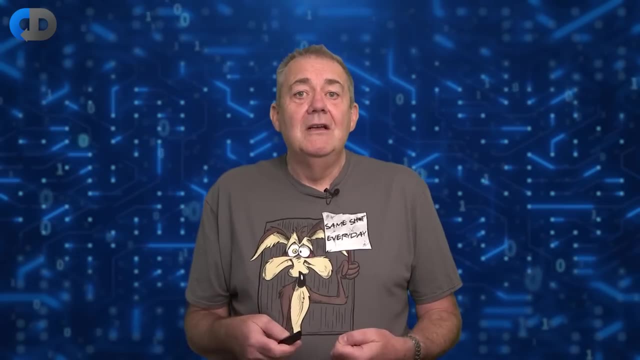 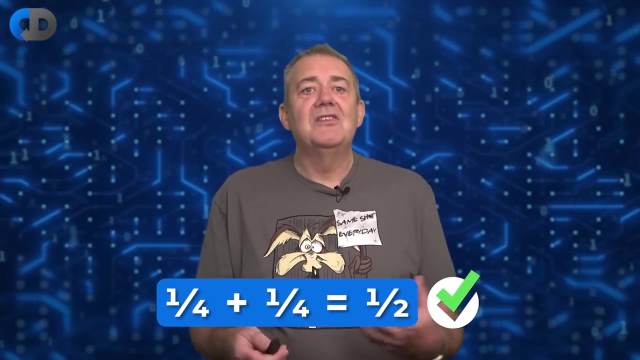 we envisaged earlier and to add the rendering of fractions with a numerator and a denominator, But we're still avoiding some of the more complex bits of adding fractions, which will presumably come later. Next we could add fractions that force us to calculate a lowest common denominator, and so on. 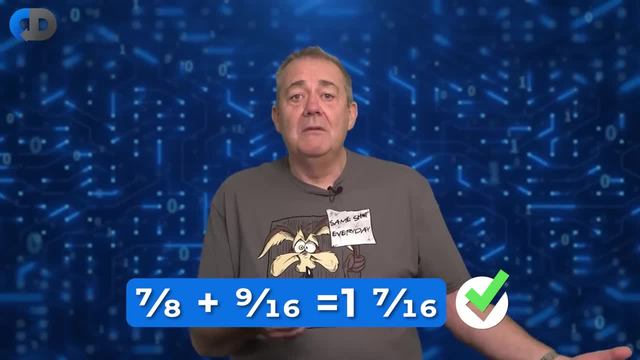 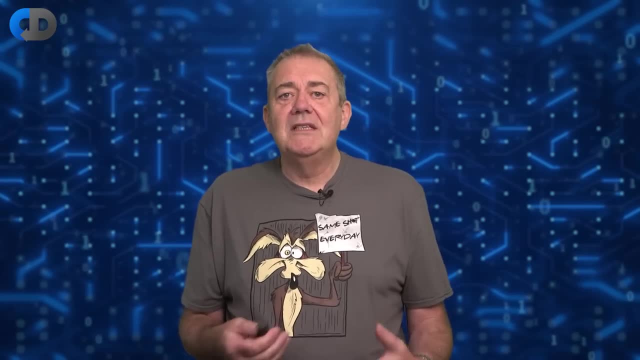 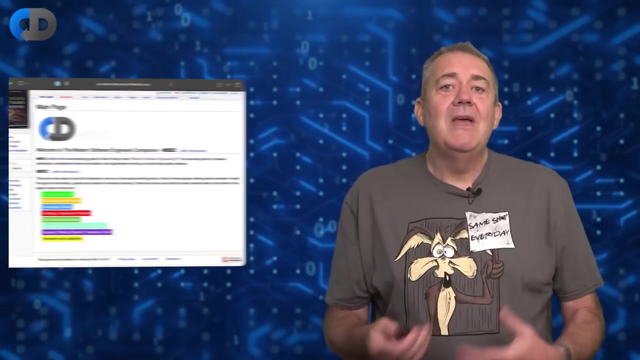 until we get to more complex cases that cover all of the types of fractions and their addition that we can think of. Let's look at a slightly more realistic, slightly more concrete example. This is some code that I am actually in the middle of writing at the moment. We have a wiki available. 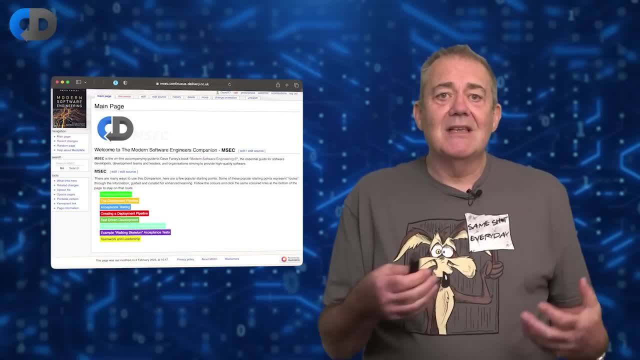 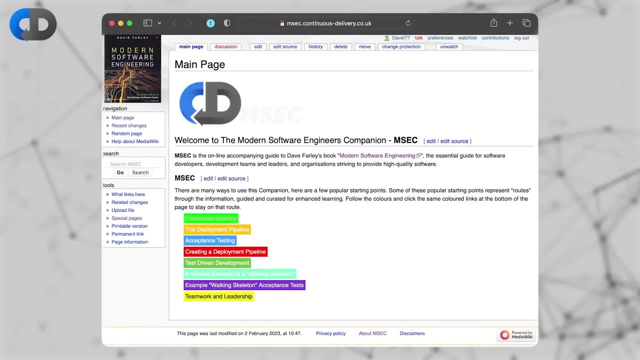 to Patreon members above Mercury level. that acts as a kind of guide and index to a lot of our content. It's called Msec. One of the ideas of the Msec is that you can follow a trail through the content to follow a strand of a particular topic. 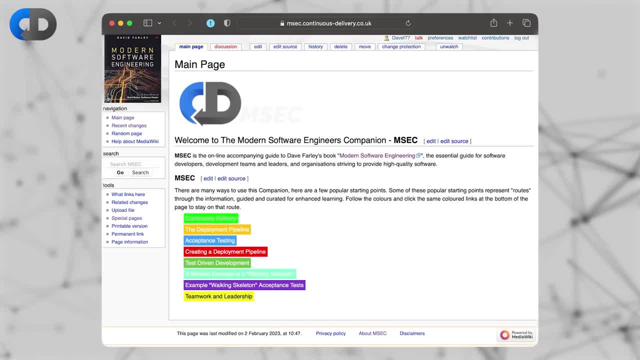 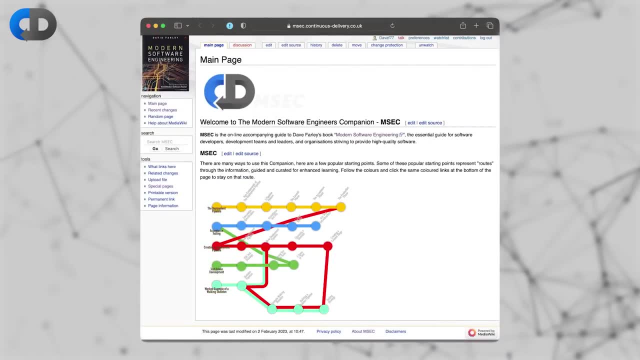 Want to learn how to build a deployment pipeline, Follow the red track. Want to learn about teamwork and leadership, Follow the yellow one, And so on. I'm playing with this idea of trying to generate a kind of tube map of for the content to replace. 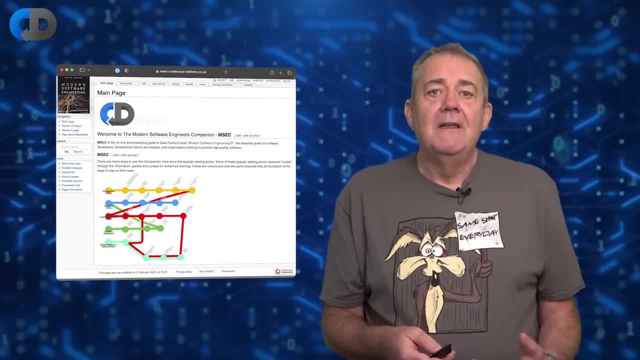 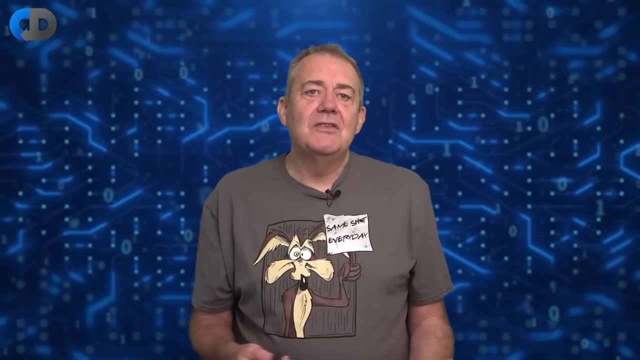 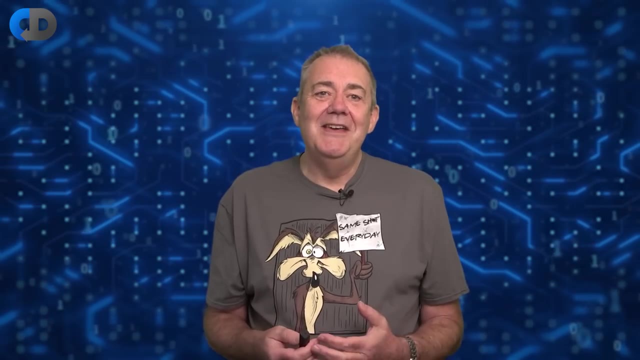 the rather manual wiki markup that we're currently using to show the tracks, So I'm playing with some code to try and get this tube map idea in place. The wiki stores content in a relational database and we version controlled it to help automate the deployment, as I hope you would expect of me. So I'm thinking about reading the content from the: 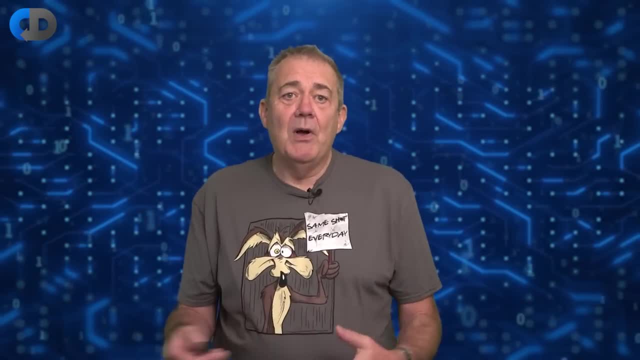 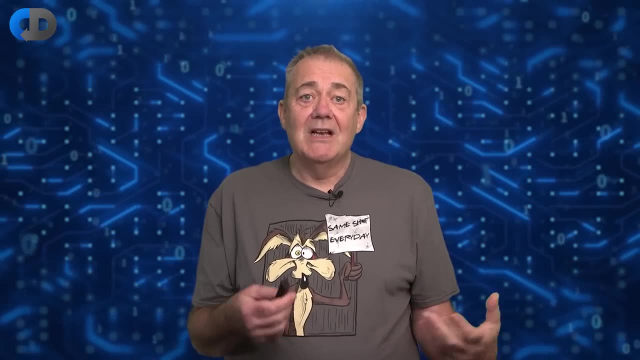 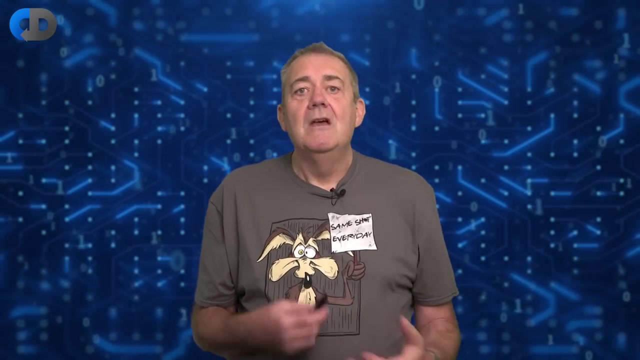 version controlled database data and then generating a map of that content. Later I will try and render page specific images of the map and markup to make the maps clickable and that I can add to each page and so improve the navigability in MSEC. A fun little project. Of course I'm using test. 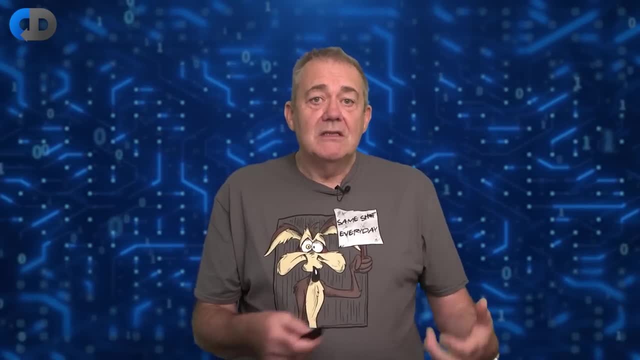 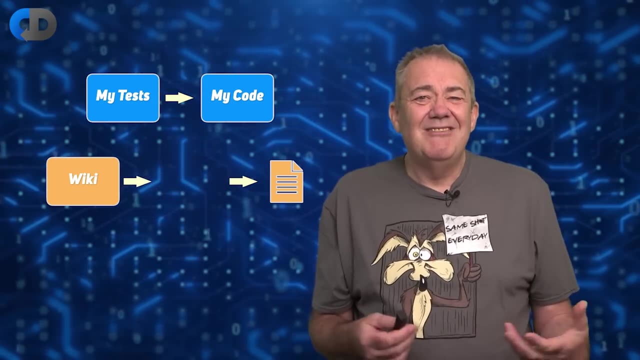 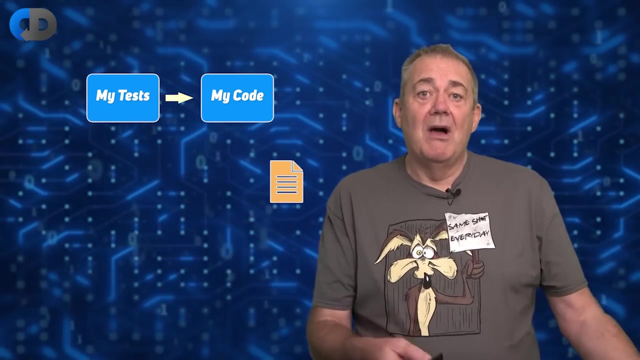 driven development. I always use test driven development And I'm exploring, so I didn't want to bake in lots of technology into my tests. I decided that for this job I didn't really need to access the real database. I can use the version controlled dump of the content and pass that as a 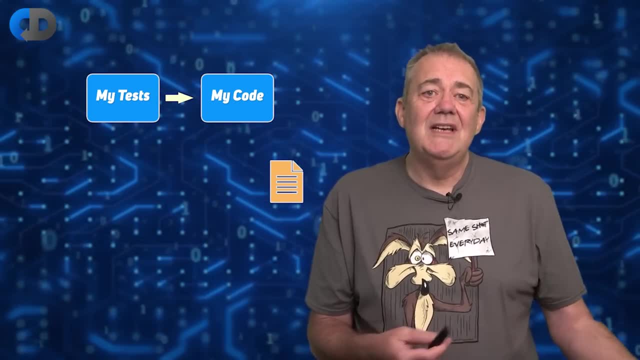 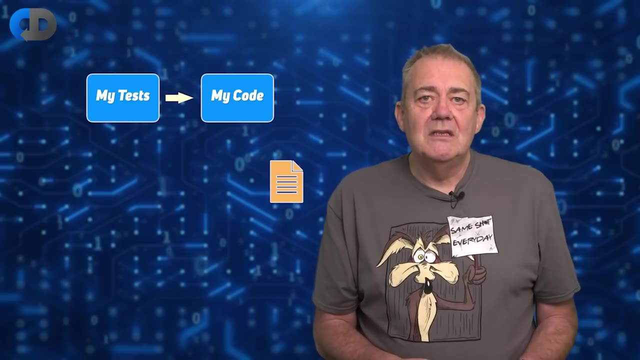 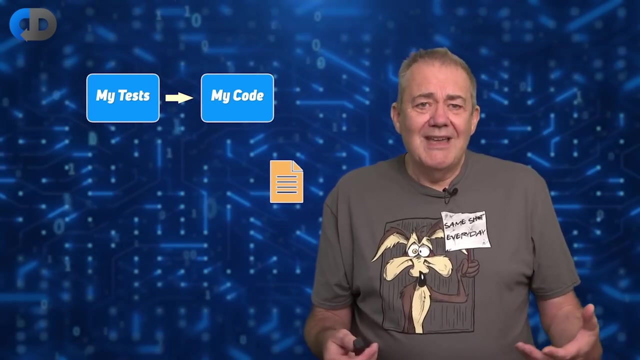 file. It's pretty basic string manipulation and so I don't really need all the complexity of dealing with SQL for this. Yes, I know this is a more coupled way to do things, and I probably wouldn't choose to do this for something bigger and more complex or less throwaway, but I can live. 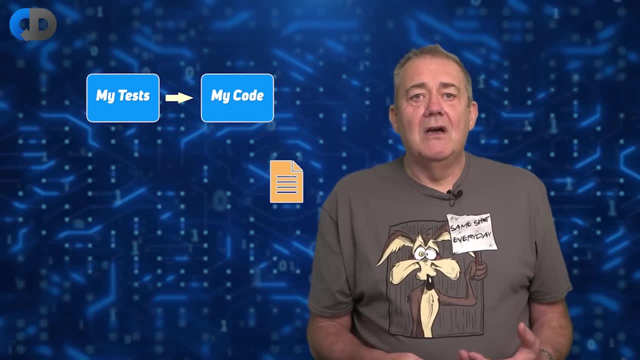 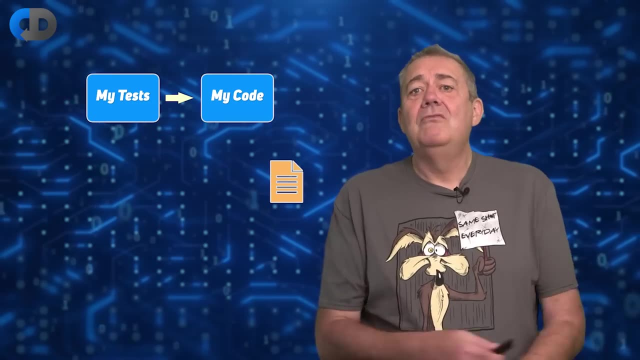 with it for this job. Basically, I've decided that I've gained nothing by using the real database here, other than making the infrastructure a bit more complicated. I don't really recommend this kind of backdoor approach in general, though, But here I think the risk I'm taking is that the 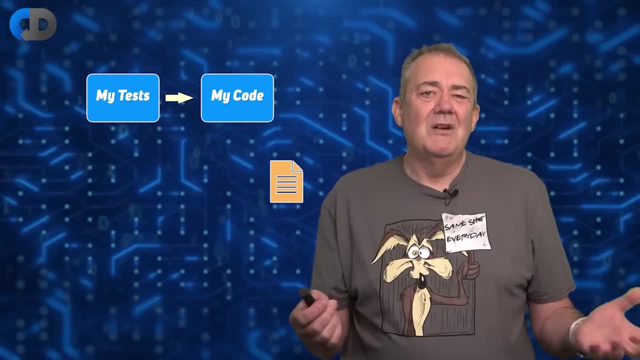 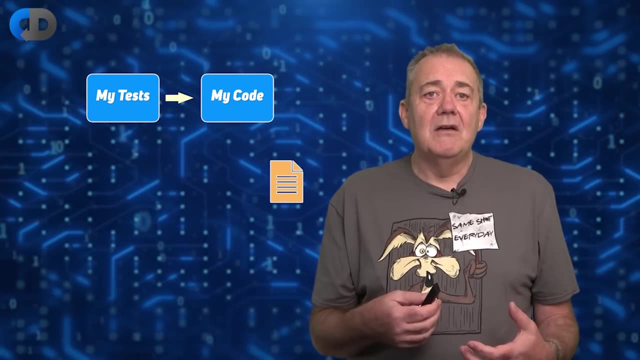 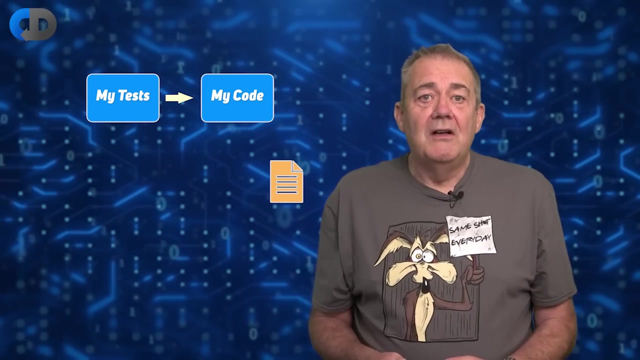 format of the SQL in the database dump changes and breaks my code. I can live with that for this case. So I decided to read the database file directly instead of accessing the data via a database. I also knew that I didn't want to be coupled to real files in my tests. I wanted to be able to 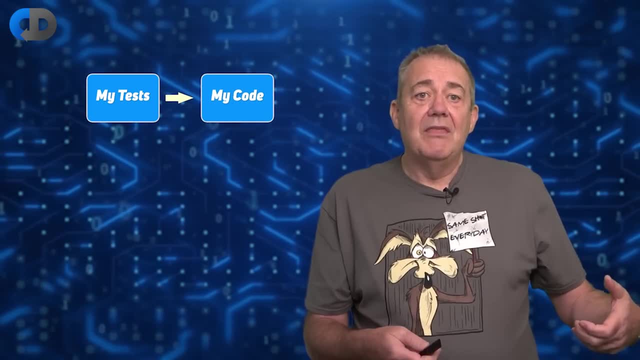 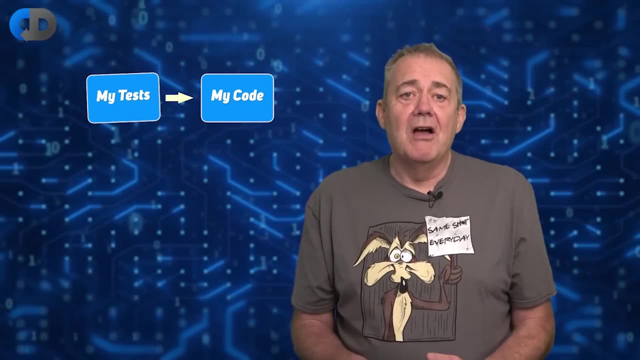 move faster than that. So I decided to assume that the content of the file that I need to parse will be presented as a string, and the starting point for what it is that I'm testing. So now my first test uses a hard-coded string. 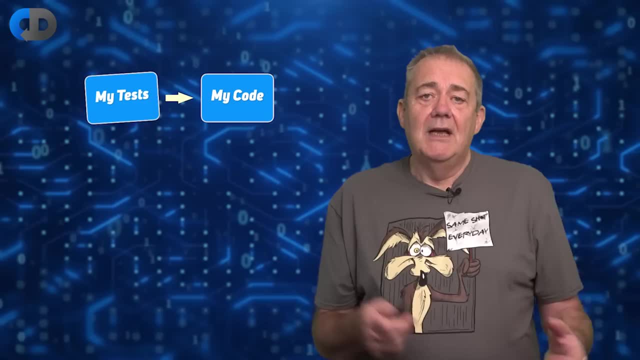 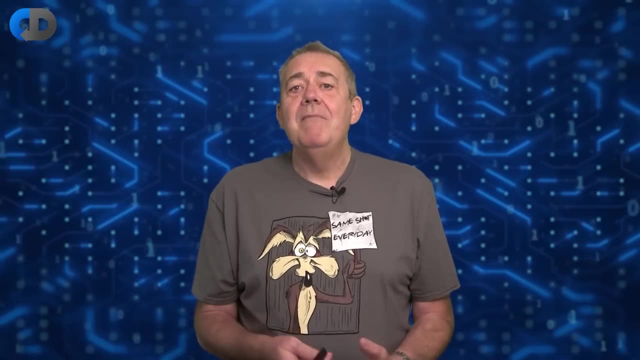 that's based on the format that will be in that file, And I've got other code that will sort out the files and provide them to this piece of code. I've made my life and my test a lot simpler as a result of these choices. My job now is simply string parsing and not 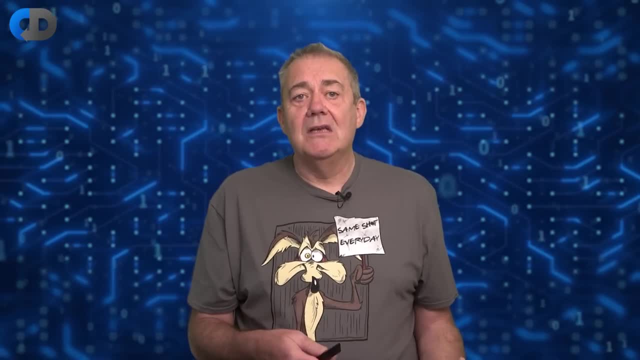 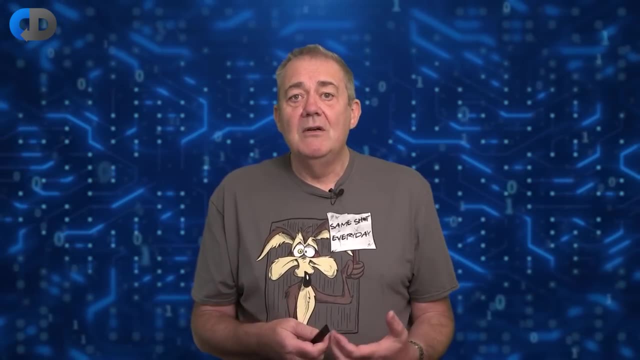 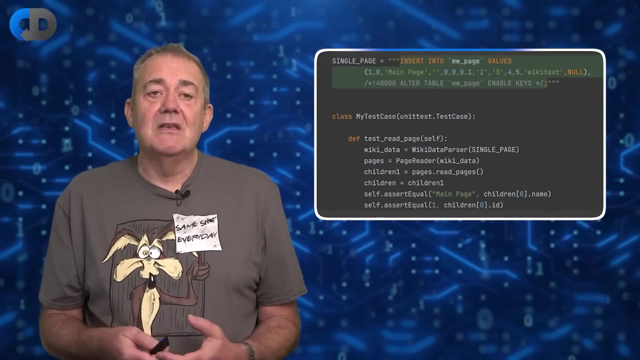 file or database handling. Now I can write tests to my heart's content without accessing the databases or files. These decisions to make my code easy to test have shaped it a bit. Once again, I've made a few starting assumptions that have shaped my design as a result. 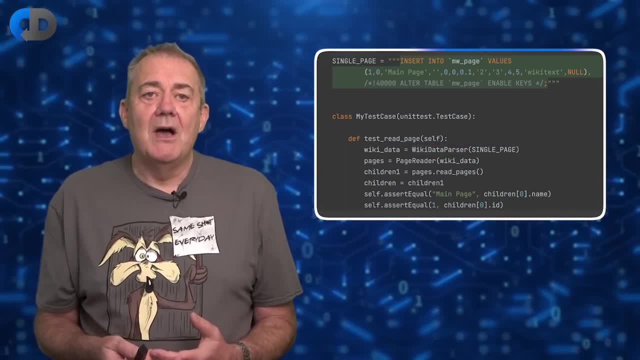 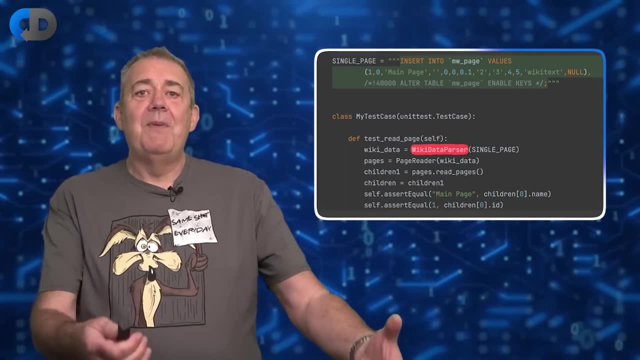 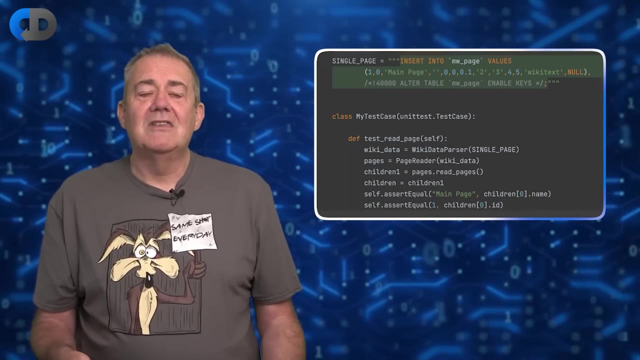 I've come up with something that I've called a Wikidata parser, which takes Wikidata as an input, the contents of the file or the database dump, and basically just filters out all of the stuff that I'm not interested in. in that piece of code It starts off at this early stage in the design. 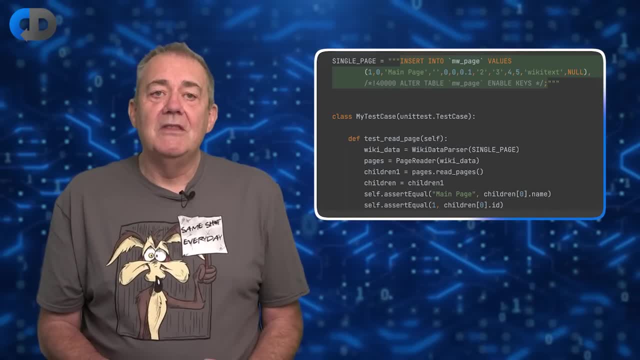 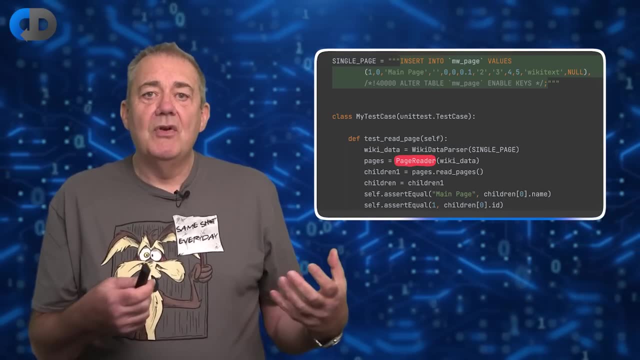 by just isolating the text that represents the page table in the database. Next, I have something that I've called a page reader. that takes a table of pages as input and creates a list of value objects, each representing a single page, But that description is with the. 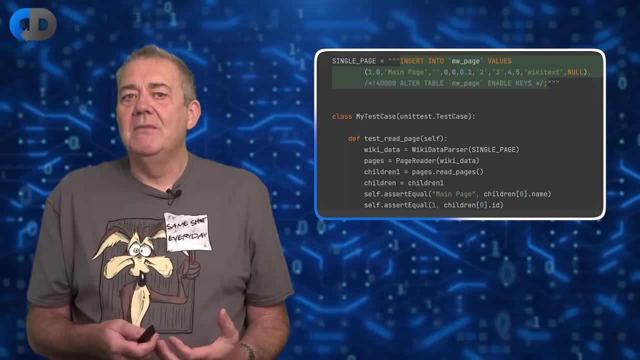 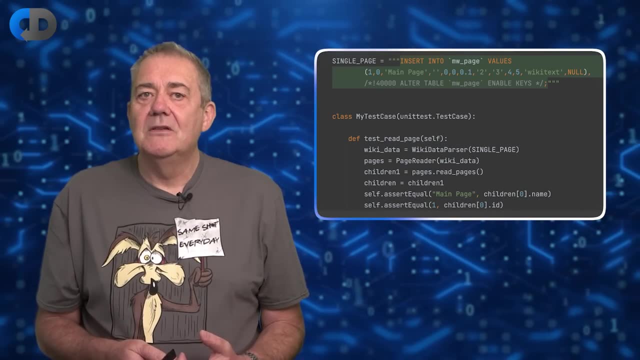 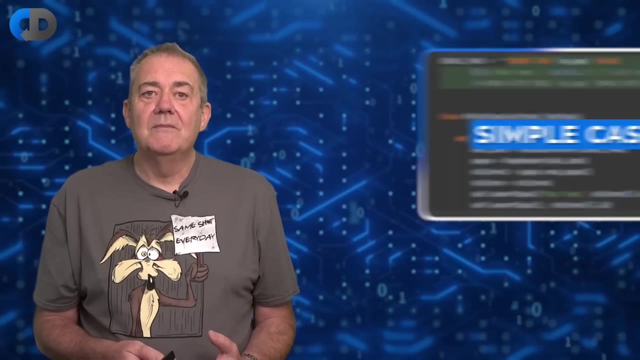 benefit of hindsight At this stage in my test-driven development journaling, actually, what I have is just something containing a single page. We haven't got to multiple pages yet. Remember, we're starting with the simplest possible case and progressing in tiny steps. 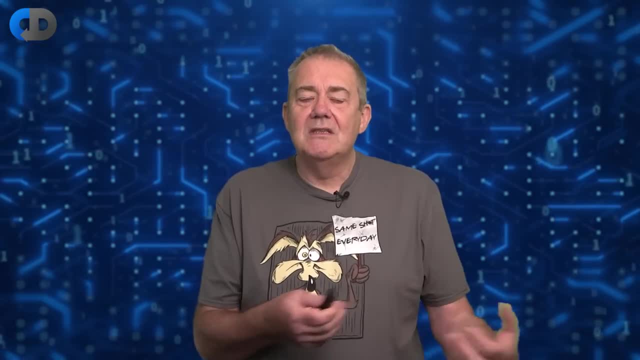 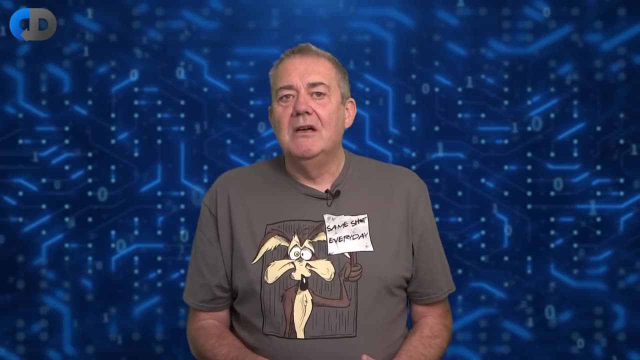 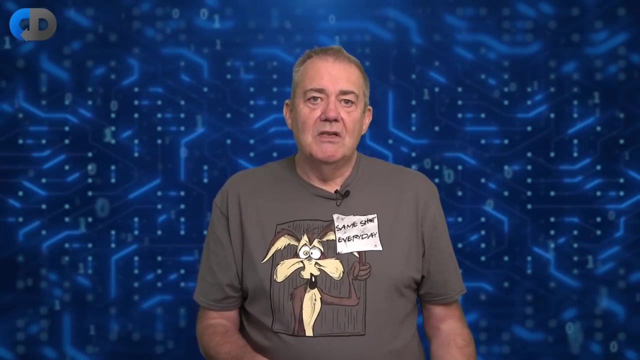 This test took a little time because I was exploring the design and how to organise the relationship between the different parts of the parsing job. but I don't think that I'm over-engineering here, because I'm not predicting where it will go next. Only that I prefer modular code with a good separation of concerns. 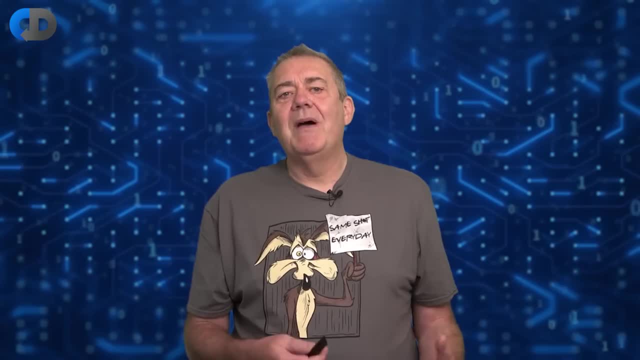 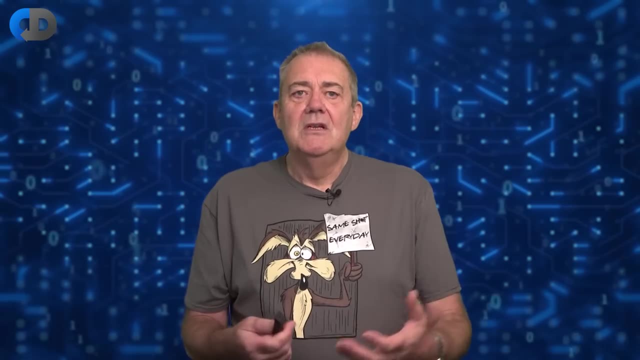 and I want it to be easily testable. The next step after this is pretty obvious. What if there are many pages? Well, in computer counting terms, two is the same thing as many. so what if there are two pages? We don't want to test lots and lots of iteration. 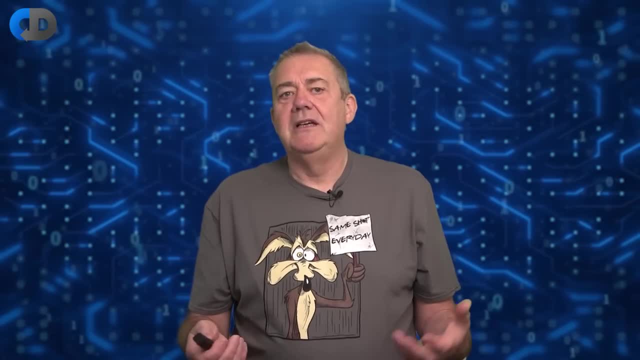 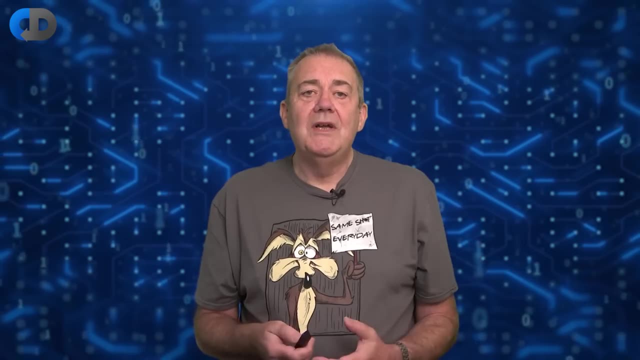 If we can loop over two, we can probably loop over two million, or at least over max int pages. It's nice to keep our tests small, fast and focused on what really matters. If you're worried about how to protect your code against looping in lists, 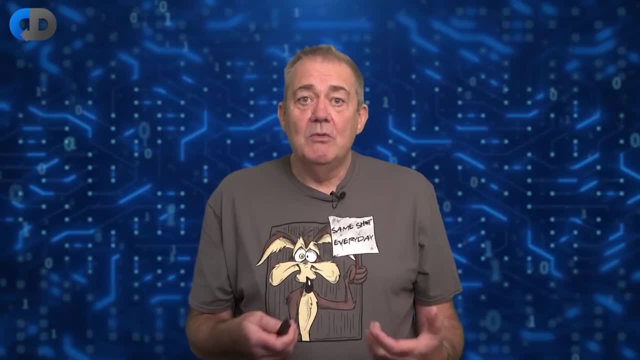 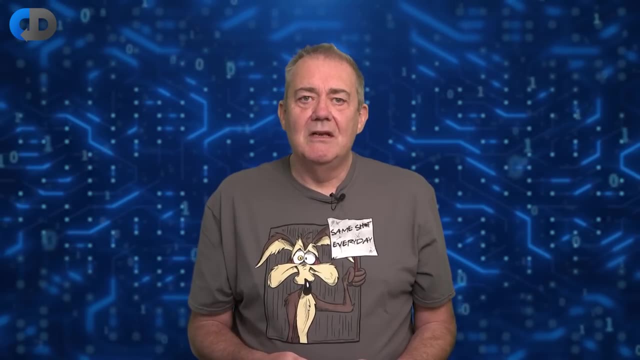 that are bigger than max int. specifically, if you're going to test two pages, specify what you would like your code to do when that happens and write that case as another test. Ideally, do this in a way that means that you don't have to evaluate it. 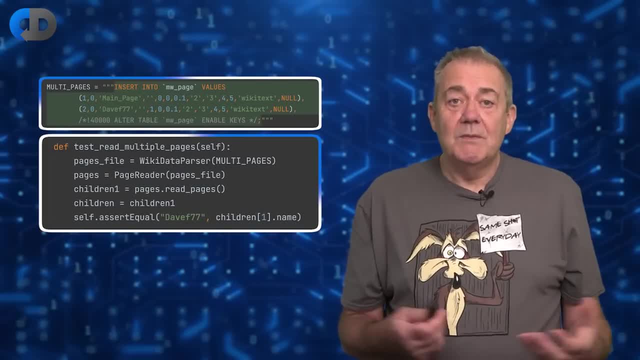 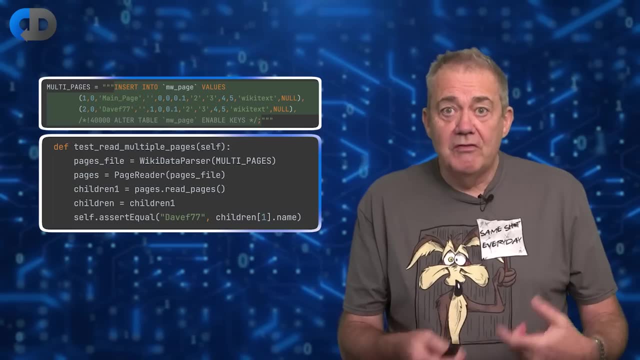 by looping over max int times. Here's my next test. It's based on a different set of data, but it's almost the same as the first. But now we're confirming that we're looping over rows of pages, two defined in the wiki data. 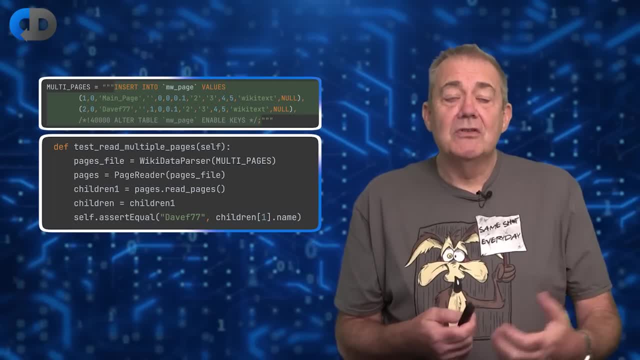 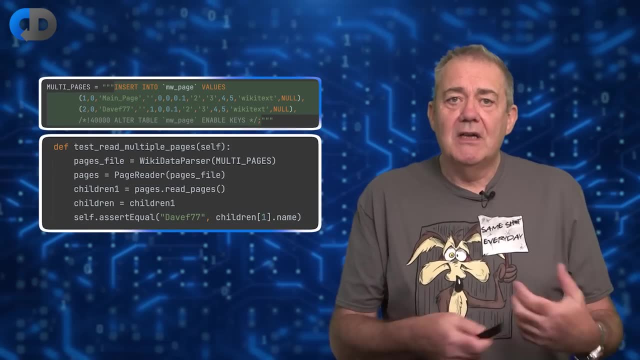 but by checking that we get the second page, not just the first Tiny tiny steps. But now I've got two, Two passing tests, and after each one my code did a little bit more. Now I'm ready for what I'm really interested in here. 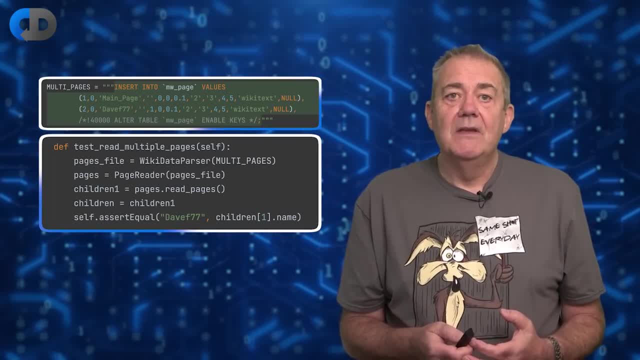 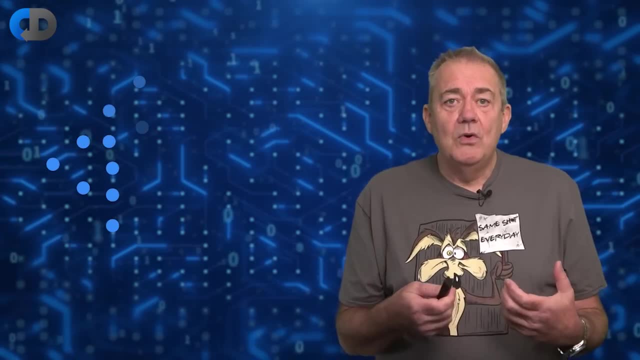 Starting to think about mapping the links between the pages. Already I've some test data for two pages, so I can probably use that again. I've decided that what I would really like is to build a kind of node tree, a graph of pages, a directed graph. 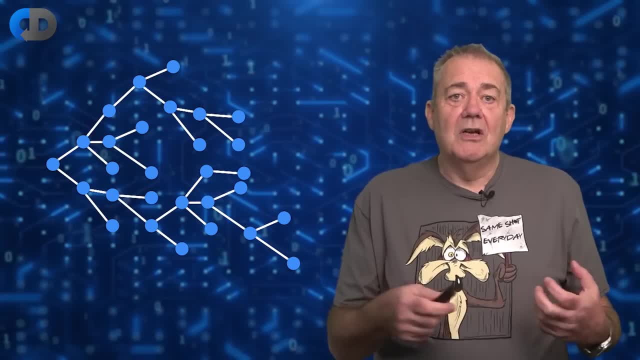 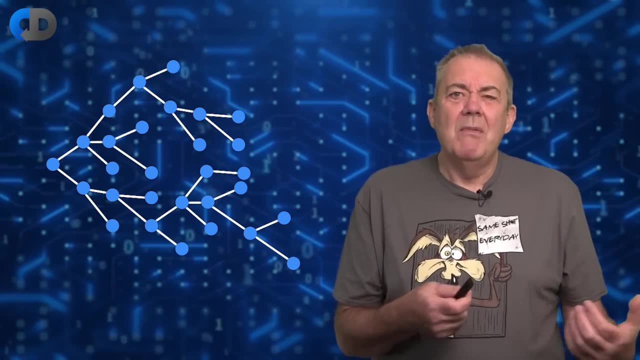 Remember. ultimately, my aim is to draw a picture of the navigation from a particular starting point. So, given my map of all the pages, I probably want to be able to define that starting point. So I'd like to request a particular starting point in the tree. 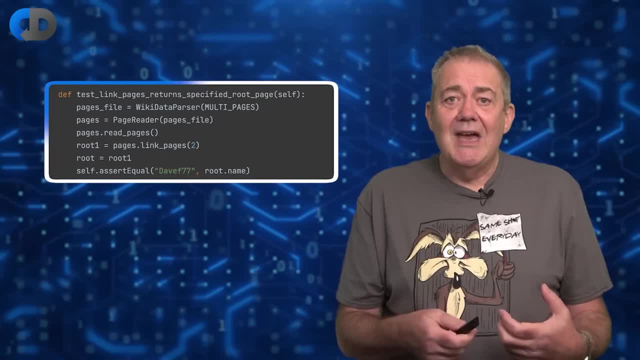 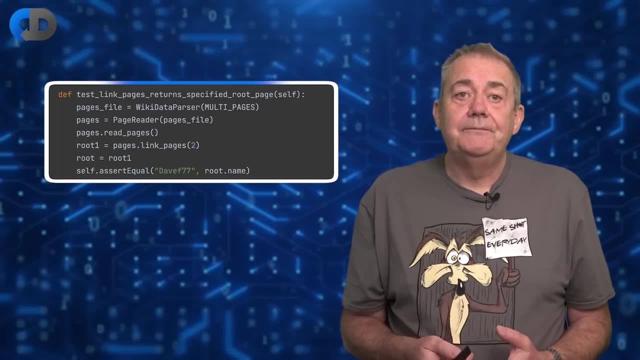 So the simplest next step that I can think of is to check that if I ask for a particular root page from the list of pages, that's what I get. This test has made me add a new method to the interface, to my code. 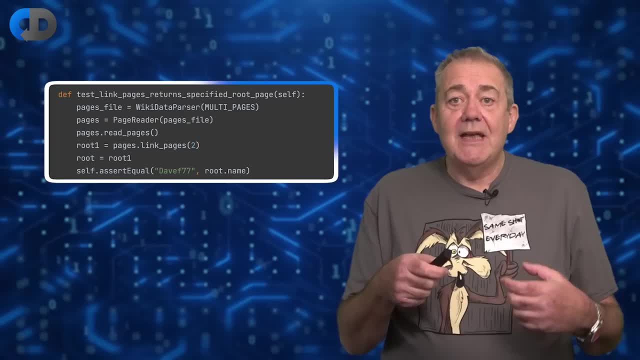 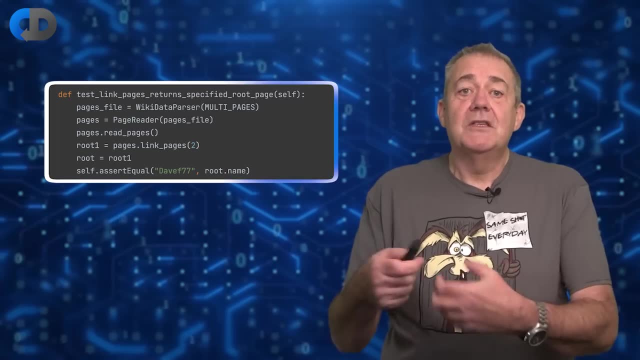 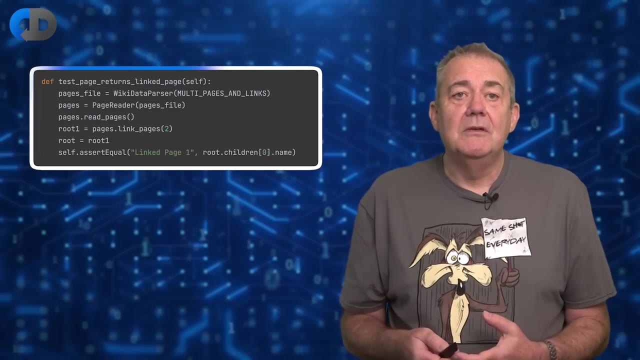 I still haven't decided how it works yet, but I've specified exactly what I want to happen in this case, and that's enough to be able to define a function that returns the specified root in that tree of pages. Next, I'd like my root page to have some children. 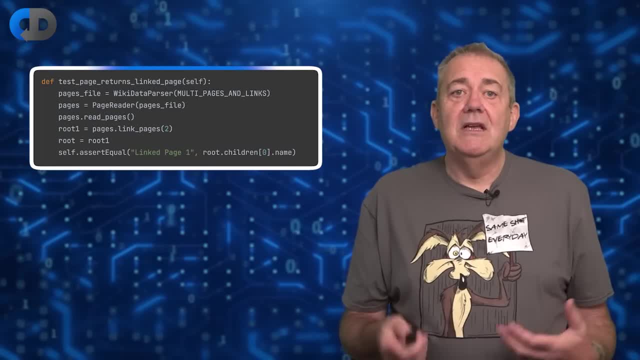 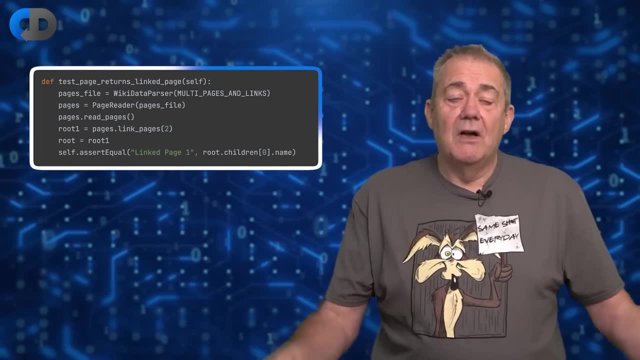 So here's my test for that And for this. I need some cleverer test data, because the links that define whether pages are related in a parent-child relationship are defined in a separate table. So here's the new data, with some links specified this time. 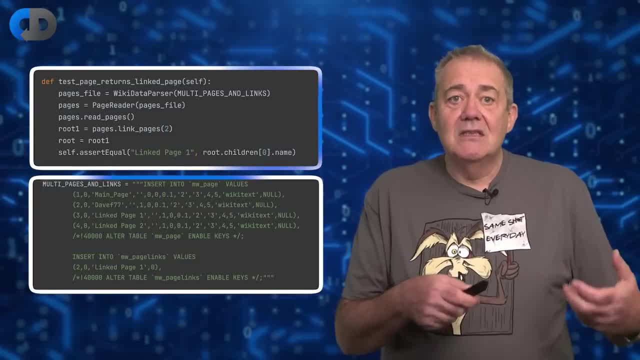 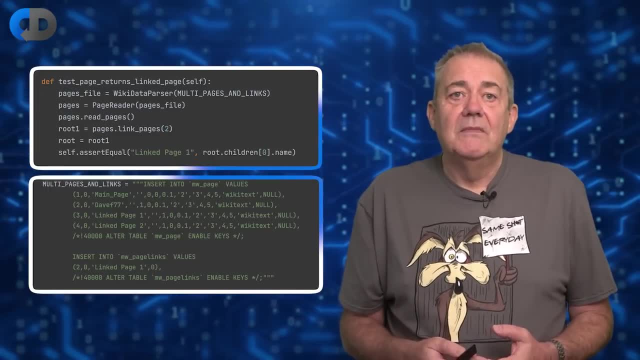 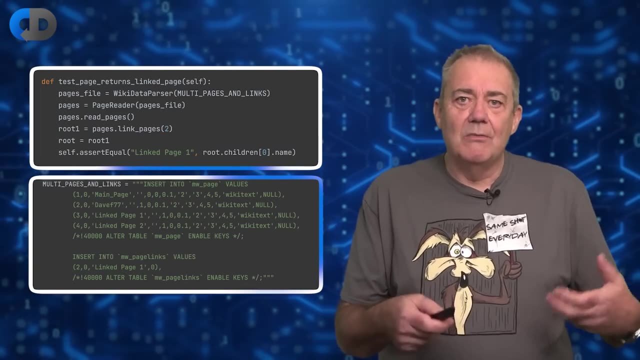 And my test once again tests the simplest addition that I can think of, So we can have one page that's linked to another. This is a small step again, but now we need to start adding a bit more complexity to the system under test to make this test pass. 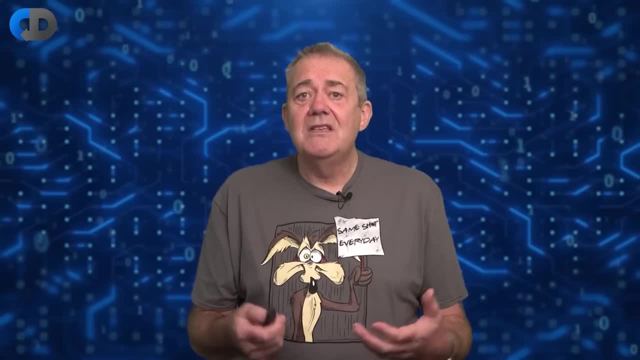 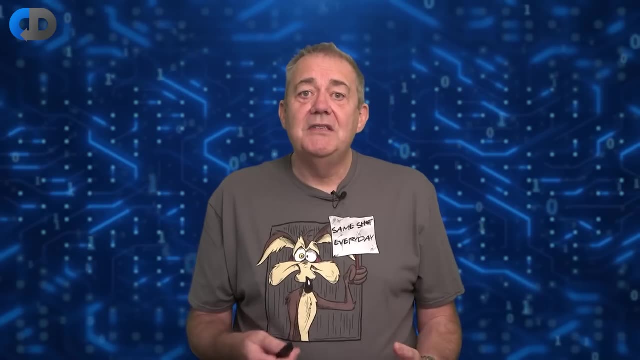 We'll need to think about this and decide how to implement it. Notice that none of my tests have any particular testing implementation detail. I could throw away all of my code and rewrite it in a completely different way, And these tests would still be correct. 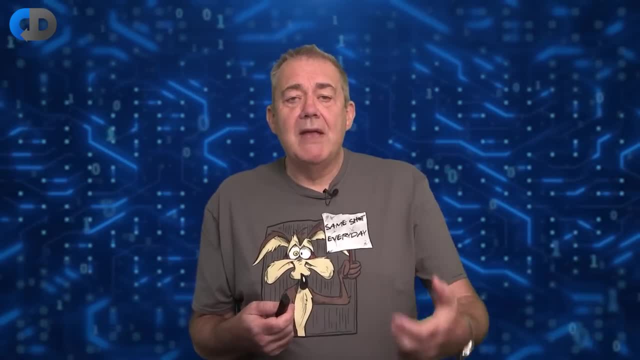 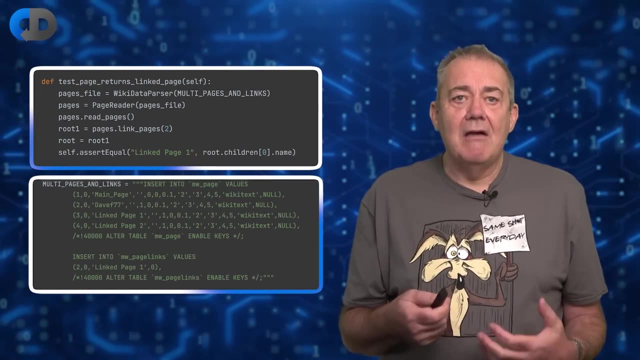 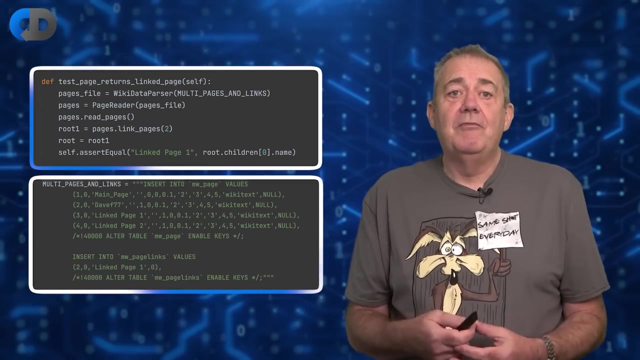 But the tests are very specific about what the code is meant to do. This is the mark of good tests, in my opinion. This latest test is now forcing me to add code to find links between pages and represent that link in my graph of pages by adding linked pages as. 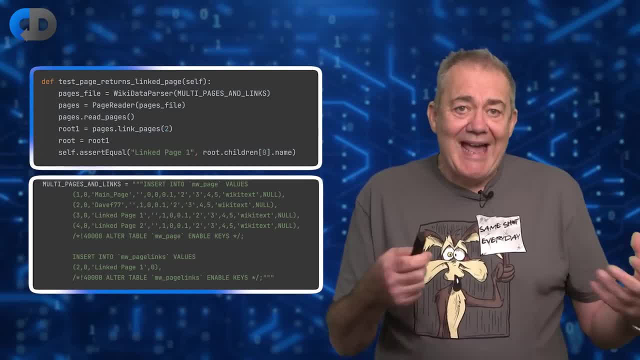 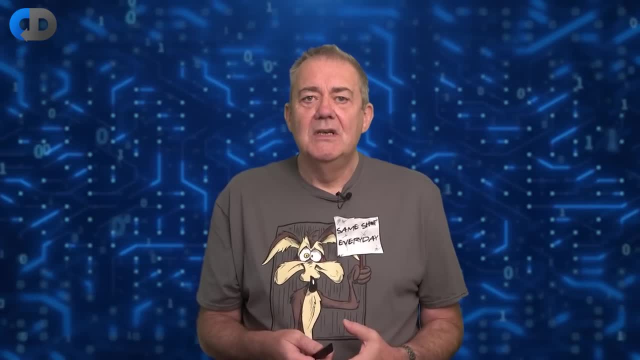 children to the current route, But it doesn't tell me how I have to achieve that, So I'm pretty happy with this. I'm not quite so happy, though, with the tests themselves. There are lots of repetition and boilerplate here, So I prefer to make them a bit more focused and readable. 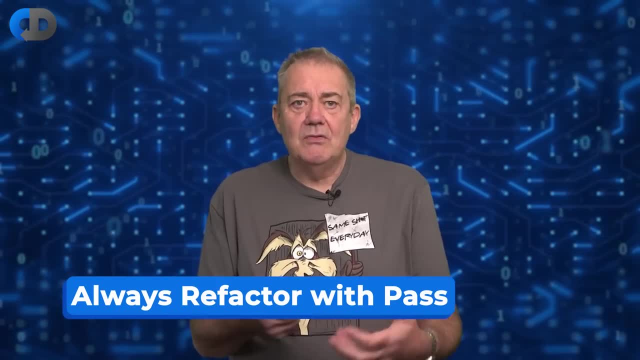 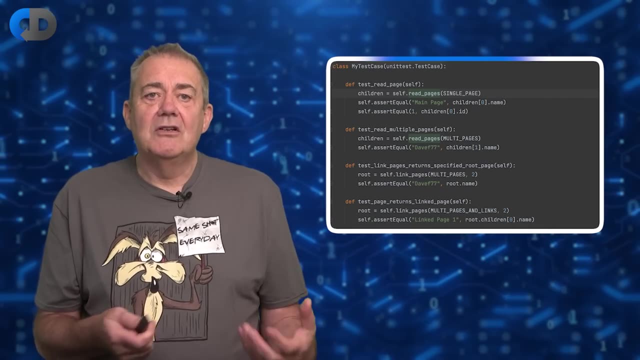 So once all of these tests are passing, remember always refactor while the tests are passing. I'm going to generalize the test code a bit. Here's what I ended up with. I've created a couple of helper functions in my test and I think 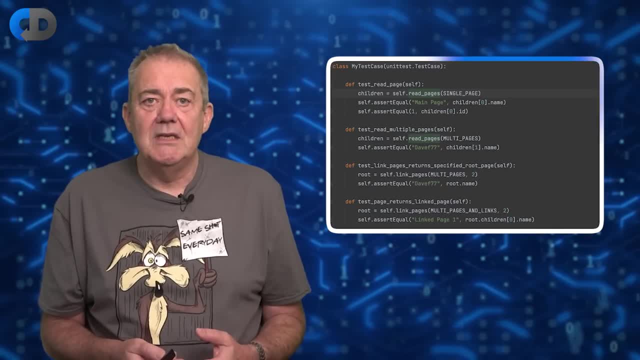 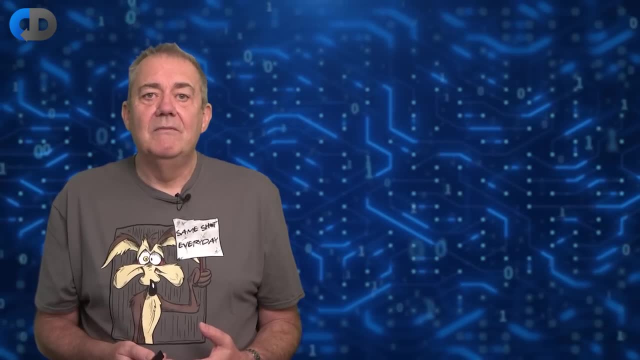 the tests now look a little bit tidier now, and future tests will be a bit easier to write. So what's the next small step from here, Once all of these tests are passing? how about multiple children? So far, we only have a single layer of hierarchy. 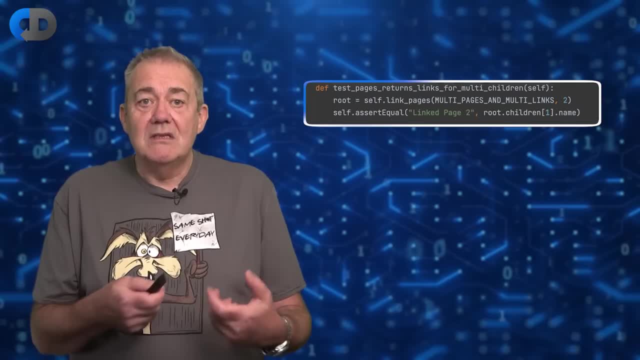 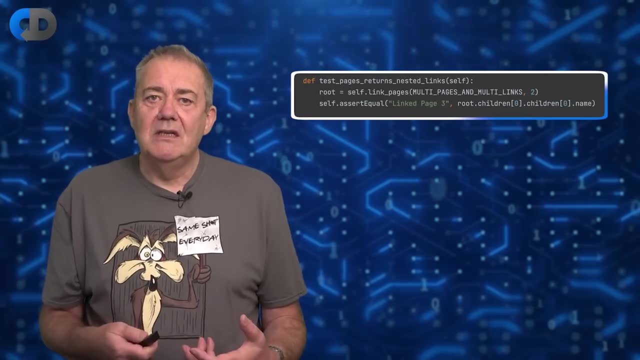 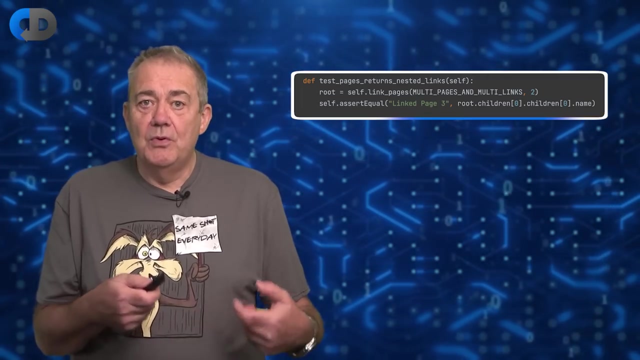 So the next obvious step after that is to build this as a proper graph of links. We need to test children, of children. At this point I decided that I'd write this as a recursive function. So now I knew that I needed another test to prove that the recursion would end.